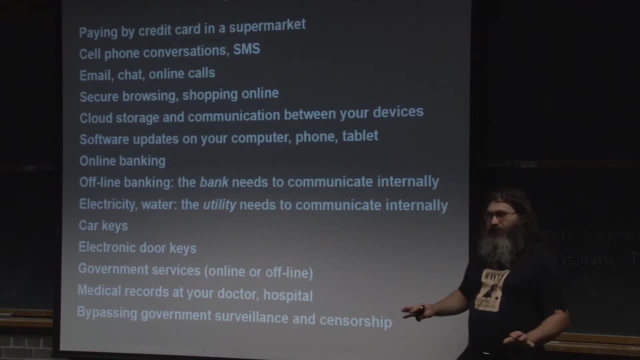 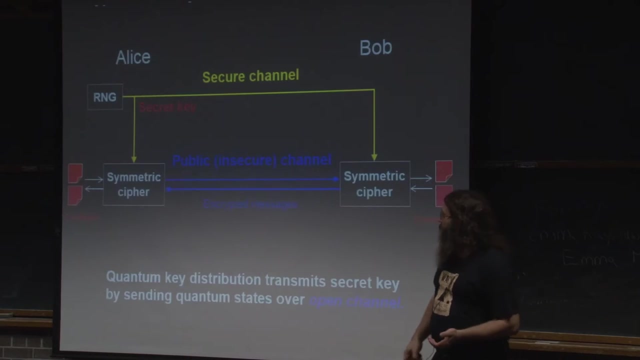 But everybody, almost everybody in the modern society uses it daily. It runs in the background. If we lost the ability to communicate securely, that will be a big step back for our society. So how to keep this ability? An important part of cryptography is encryption. 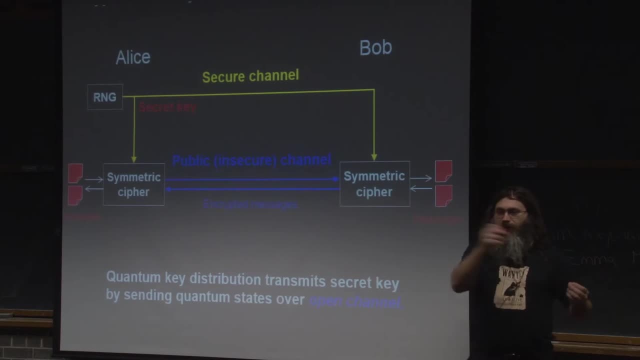 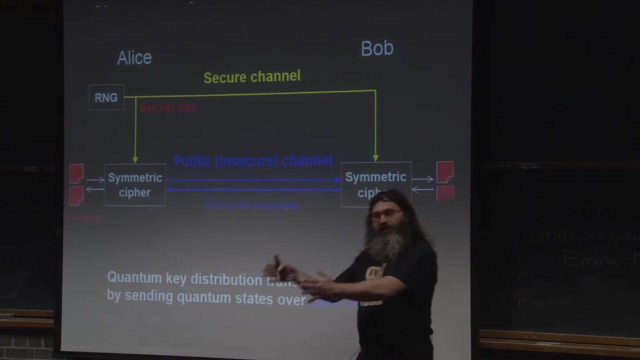 Secure communication allowing you to encrypt a message, transmit it over the communication channel and decrypt, And while the message is in transit in the communication channel, somebody trying to read the message can't figure it out. It looks like garbage, But the receiver will successfully decrypt the message. 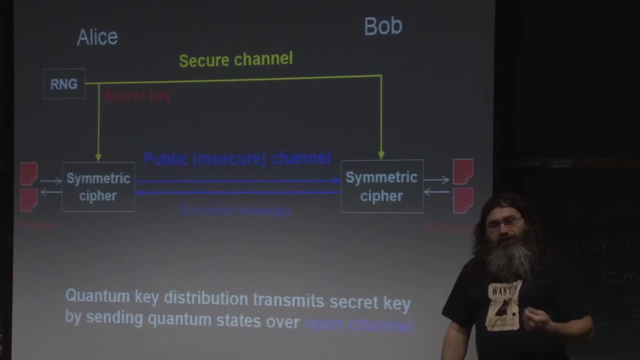 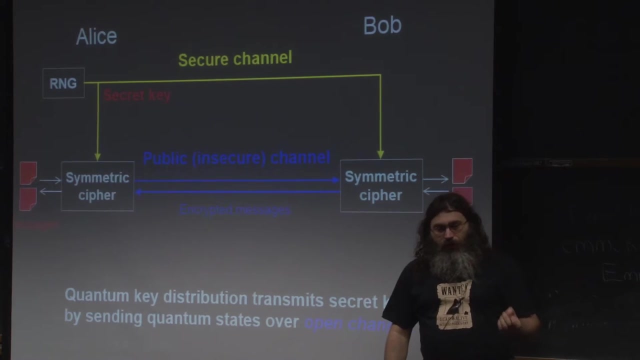 A typical encryption and decryption scheme consists of sender Alice and the receiver Bob. Before they can communicate securely, before they can actually transmit the encrypted message, Alice and Bob have to transmit between themselves a secret key, a random secret key. Once Alice and Bob have each a copy of this key and they are sure that nobody else has this copy, 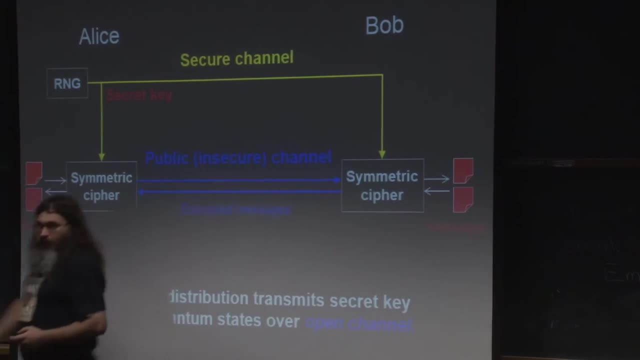 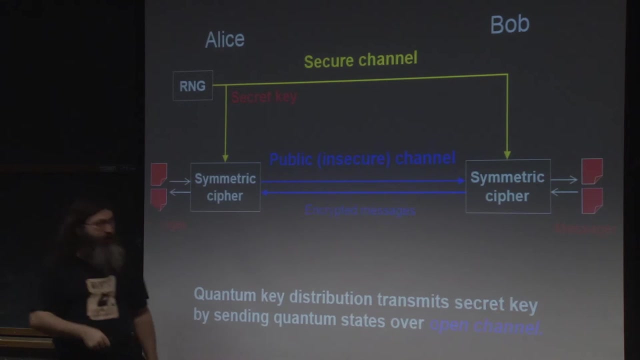 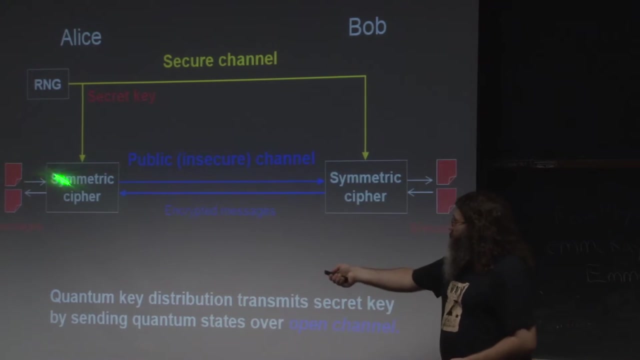 then they can use the secret key to encrypt the actual secret message, transmit it in encrypted form over the communication channel and, using the same key, decrypt this message. This encryption and decryption is the easy part. There are good ciphers, good hack-proof, hack-resistant ciphers that allow to do that. 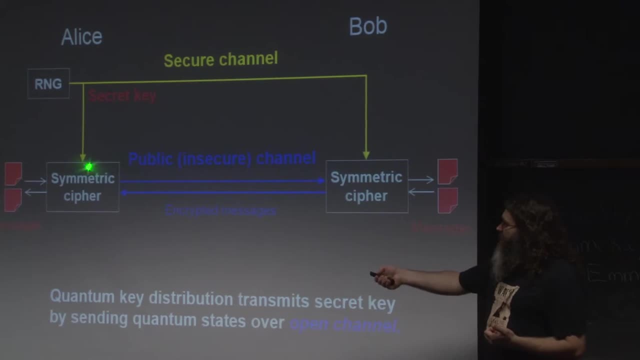 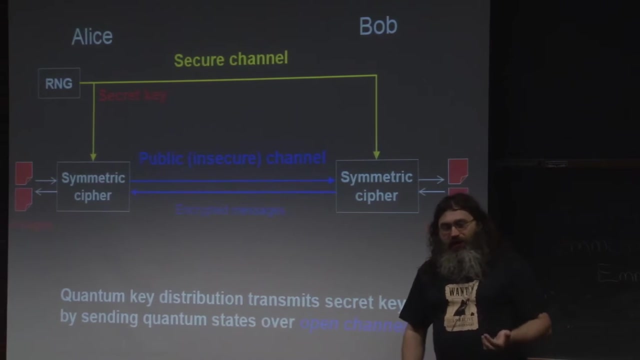 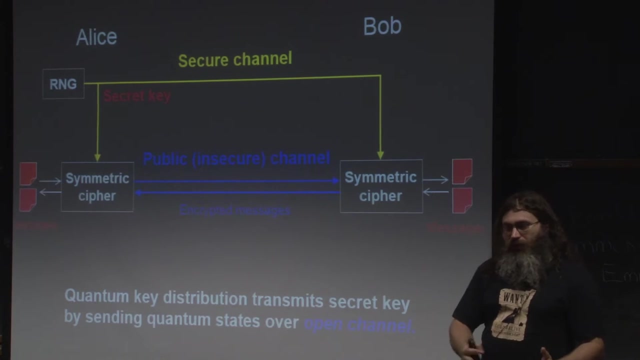 The difficult part is to share the secret key, the secret key between Alice and Bob, Because if you do it over a classical communication channel, any classical communication channel can be eavesdropped and somebody can make a perfect copy of the information going on the communication channel. 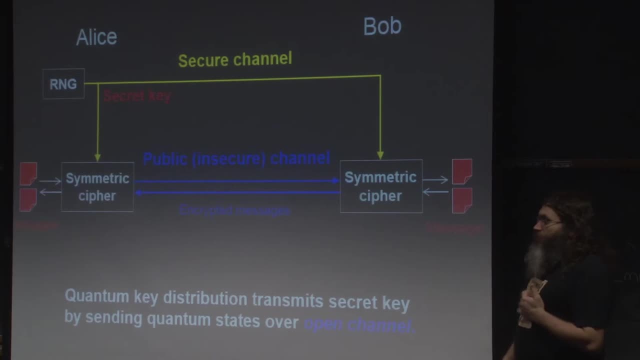 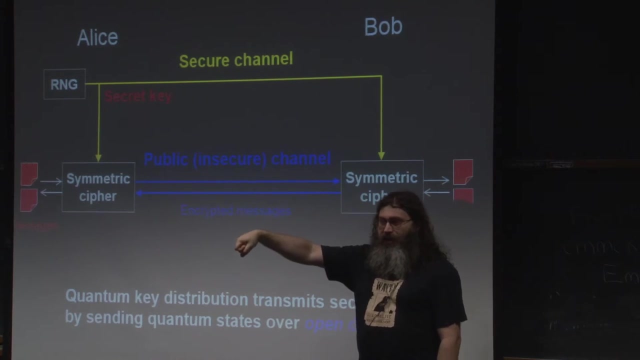 That's the classical information Today for most well, for more secure communications. today the copy can be distributed by a courier, somebody physically carrying a suitcase, a hard drive or a USB key and delivering a copy of the key between two users. 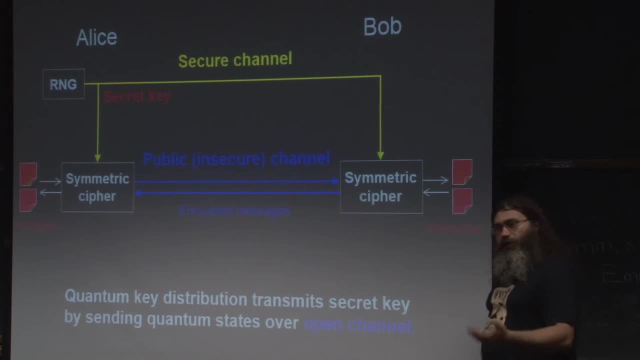 And this is used for diplomatic communication, for spies, for more secure corporate communication. but this is of course expensive, impractical and this can only be done between a limited number of users. So this physical distribution method doesn't scale to a network. 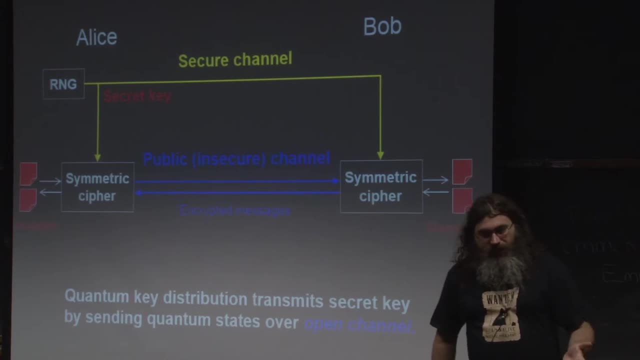 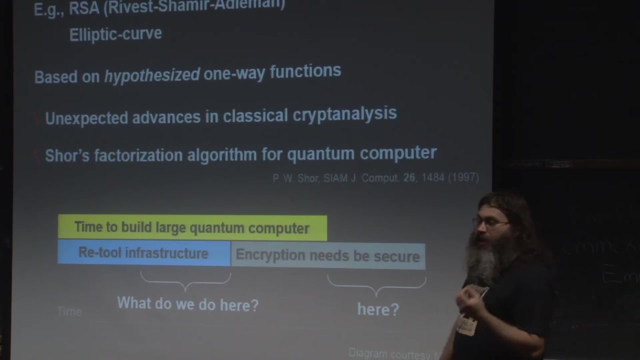 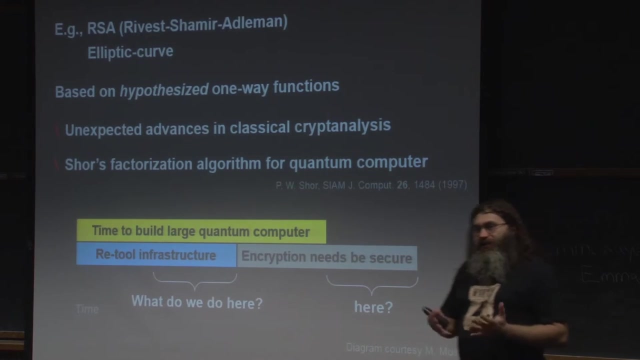 For most secure communications today on the Internet. what is used instead are mathematical ciphers that allow to distribute the key, so-called public key cryptography. Those are mathematical methods which are based on mathematical assumptions. The assumptions are such that there is a mathematical function. 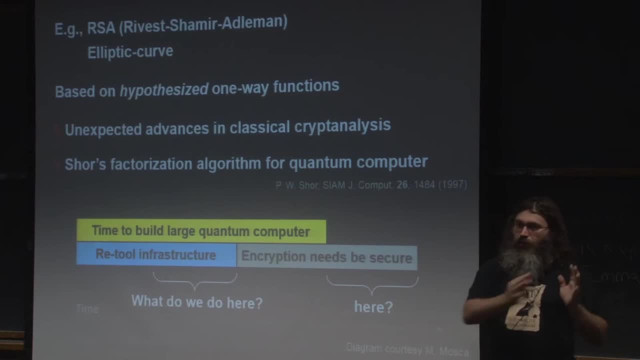 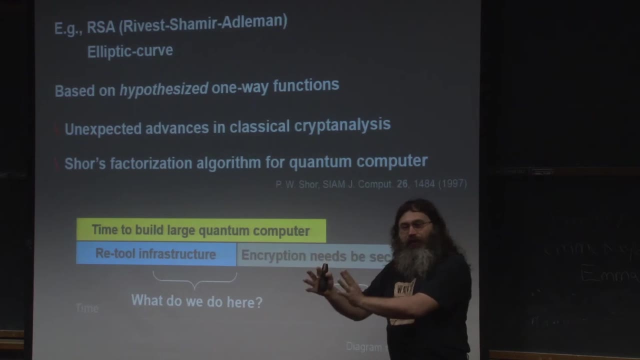 which is very easy to compute in one direction, from the argument to the result of the function, But very difficult to compute in the reverse direction. So if you have the result of the mathematical function, it is assumed to be very difficult to find out. 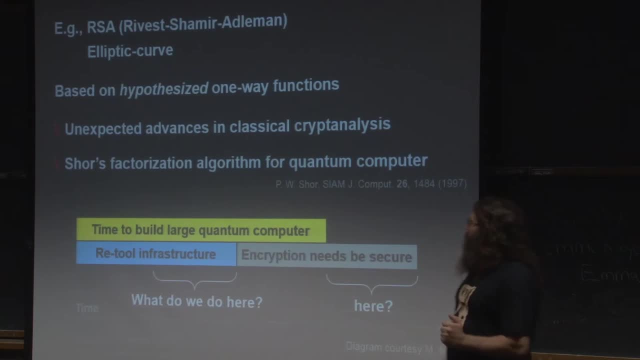 what the original arguments are: so-called one-way functions. Their existence in mathematics is not proven, It is just conjectured. The well-known ciphers are: RSA, Revis, Shamir, Adlyman, public key, cryptography or, if you use Blackberry, 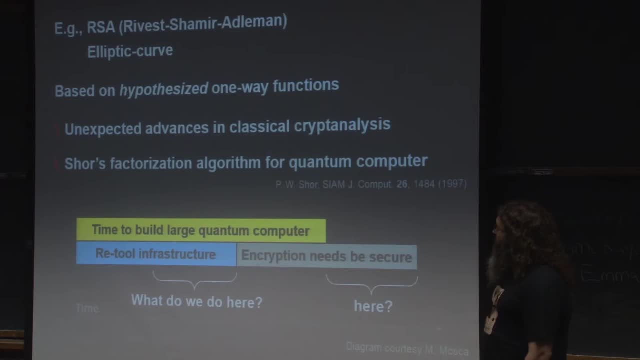 you are using elliptic curve cryptography and the problem with those mathematical ciphers is just dot. Nobody really knows whether they are secure or not, because nobody has proven that they cannot be cracked. Furthermore, we know that when we build a quantum computer, 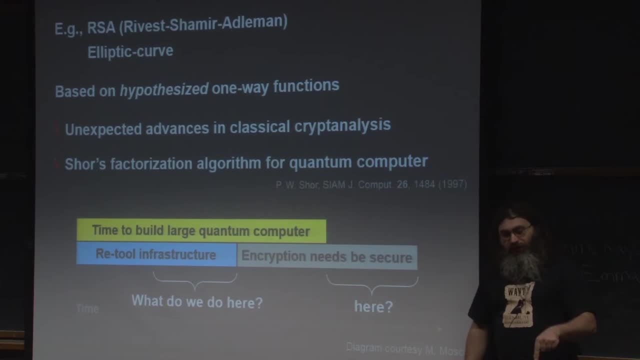 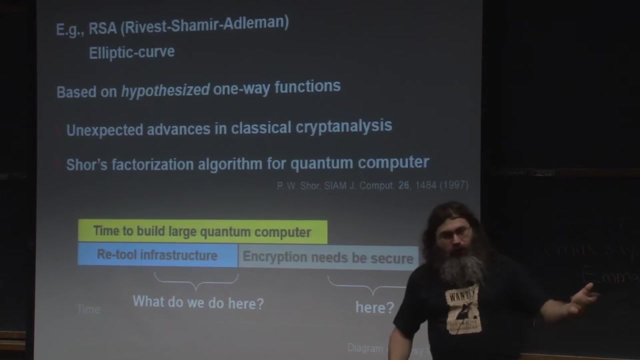 those ciphers will be cracked because there is an algorithm for a quantum computer, Shor's factorization algorithm- that allows you to crack both types of public key cryptography. So, in essence, if we at the Institute for Quantum Computing had a quantum computer today, 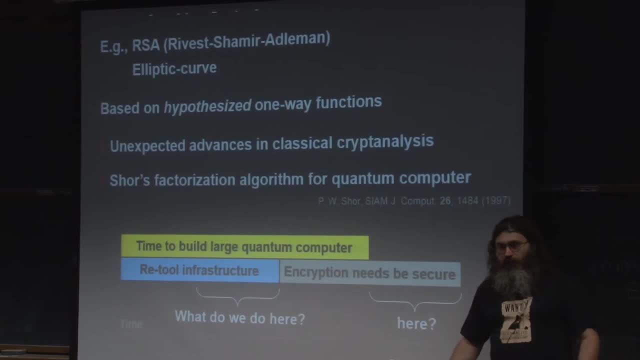 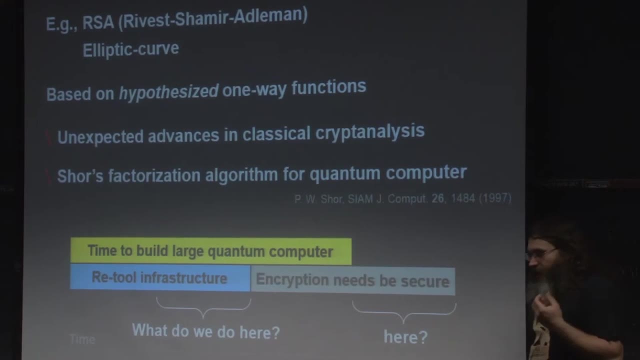 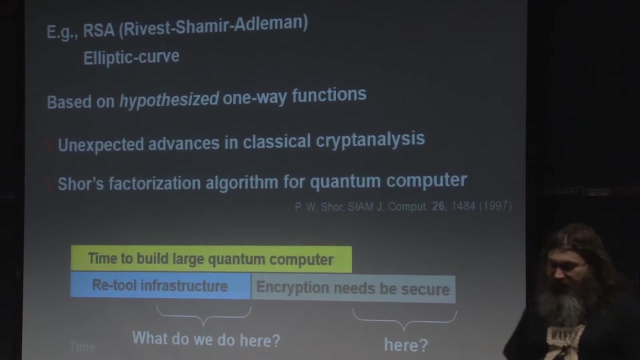 all. the Internet will become insecure in an instant, because this is the encryption used on the Internet and there is no ready alternative for it. So the aging mathematical ciphers have to be replaced by something which will be resistant, at least be resistant to a quantum computer. 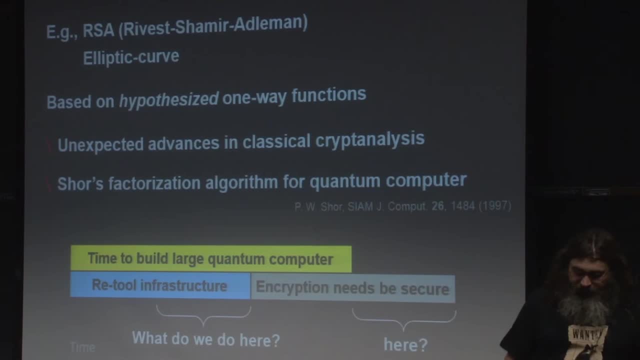 And we have to look for alternatives. The important question is how urgent this is. We don't have a quantum computer yet. If you ask my fellow professors at the IQC, they will give you different answers. when the quantum computer will be built? 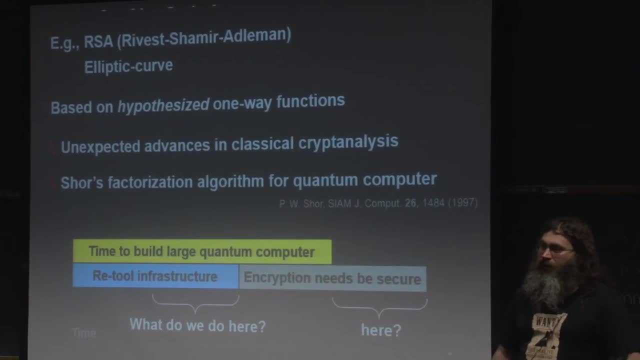 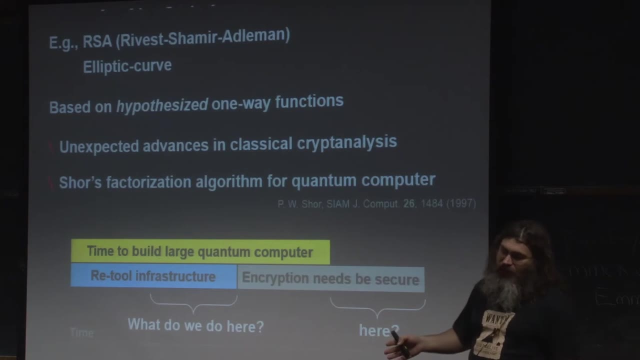 They range from next year to never. If you, yes, if you average between dots, we can arrive at something like 15 years average answer. So say it takes a number of years to build until we actually have the quantum computer. Can we just sit and wait? 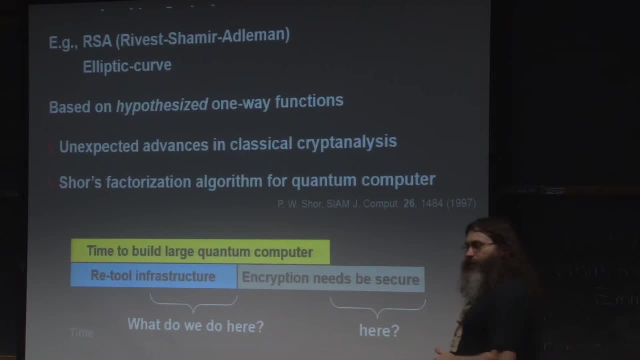 and when the quantum computer is built, go and update our current cryptographic methods. No, Because, first of all, the information you encrypt today has to stay secure for some length of time. Well, if this is your email or a credit card number, it probably doesn't have to stay secure for long. You will get a new credit card next year- But there are many types of communication which have to stay secure for long: Medical records, banking records, certain private communication, commercial secrets, government secrets. 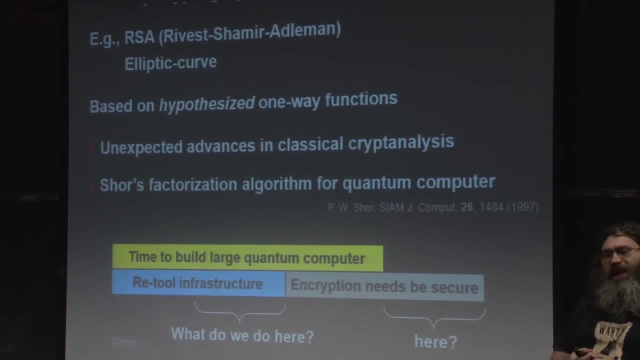 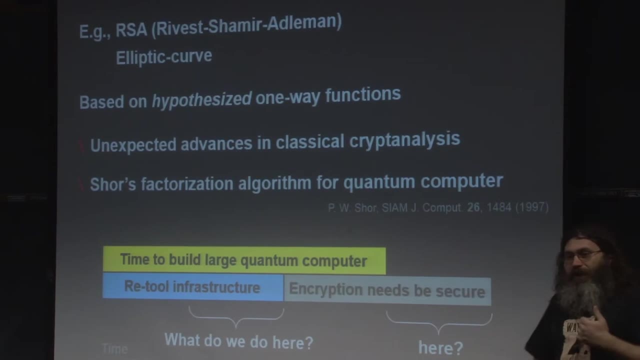 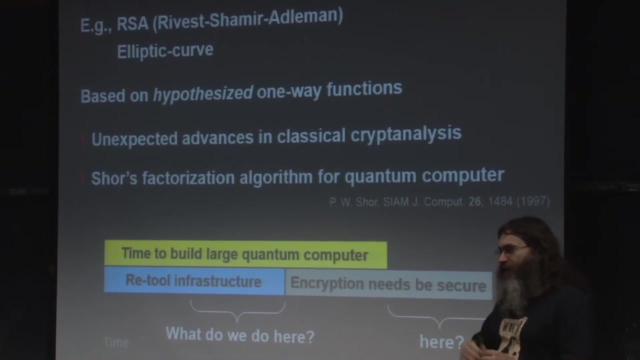 military secrets. They have the lifetime of decades. So many important communications have to be stay secure for long. But face it, when we have the quantum computer we can decrypt all the classical communications retroactively. So we can't crack them today. 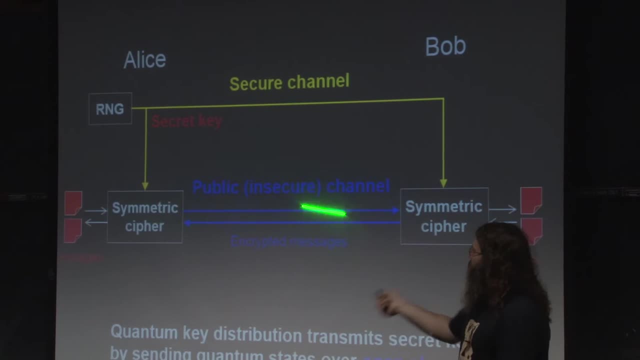 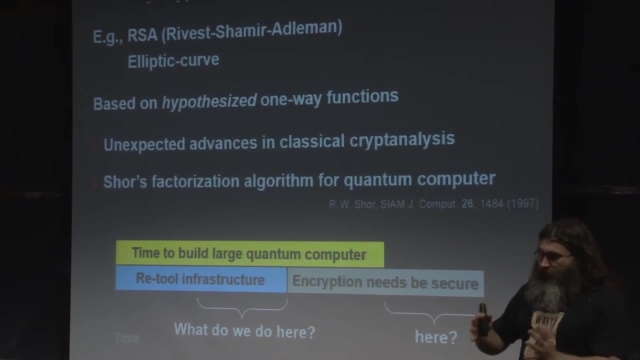 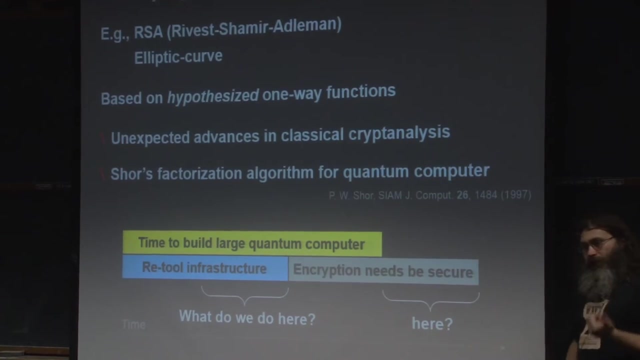 But we can record what's going on in this communication channel and in that communication channel And then later when we have the quantum computer, then we can run our quantum computer and crack and read all that retroactively, So the lifetime of our information. 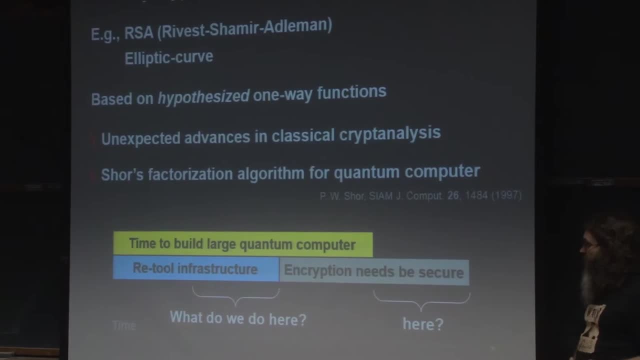 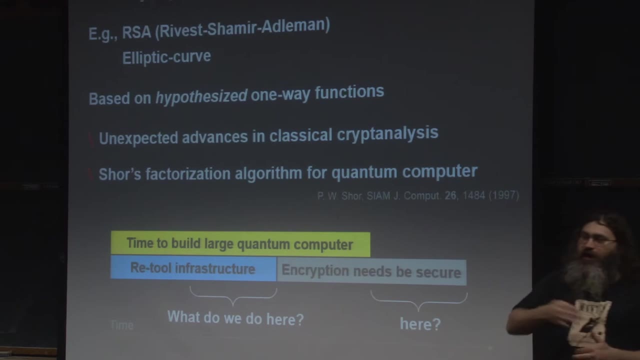 is how long the current encryption methods have to last. And second question is: once you have the technology ready, how long does it take to update the technology, To actually replace all the devices, replace all the algorithms, And that also takes a number of years. 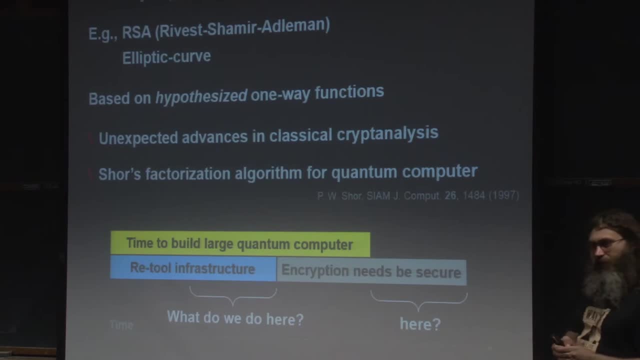 So, in fact, we think we are already too late to think about this question. Well, this is human nature. We are not very good at long-term planning, But I think this is the situation And it will be a big fun to watch the press. 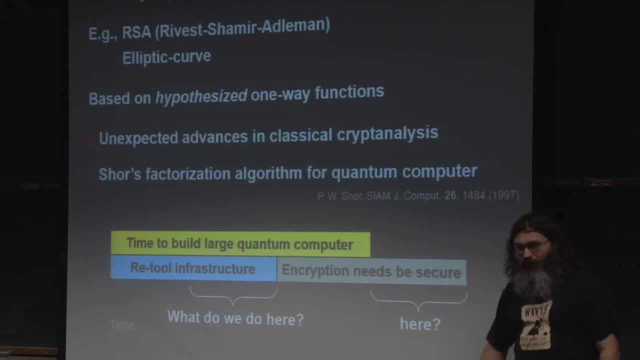 and the world react when we have cracked our classical cryptography. but nothing is ready yet. But good news is people are working on replacement for current cryptographic methods. There is a movement in the mathematical community to try to find algorithms which are resistant to our quantum computer. 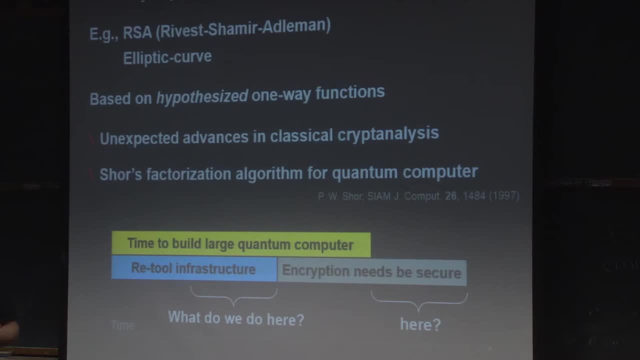 So right now at the AQC there is going a conference of those mathematical cryptographers who are discussing that question, But as I understand, they are at a relatively early stages in that discussion. So no algorithm, no such algorithm. 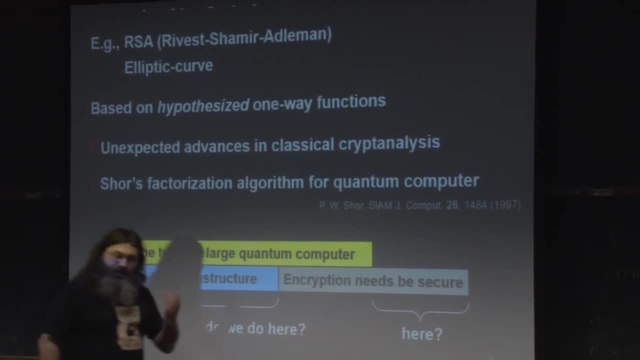 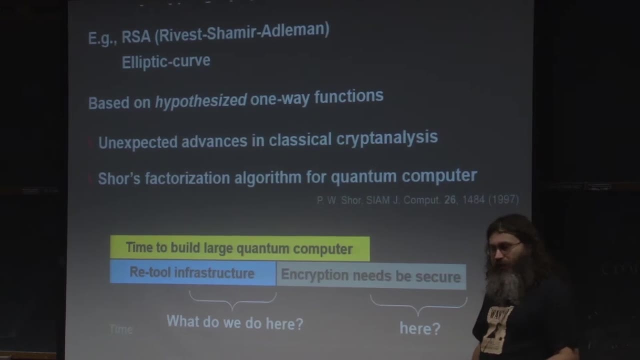 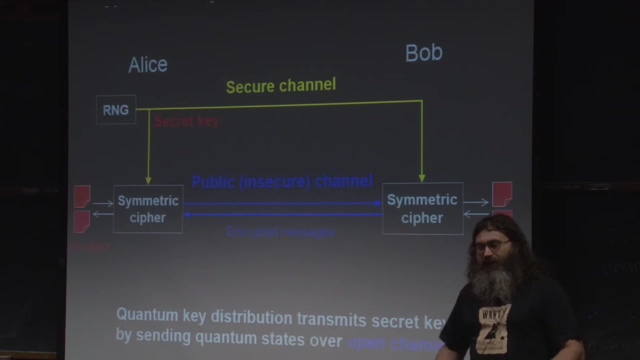 is yet ready for deployment. And there is another technology, quantum cryptography, which is more ready for deployment and which is resistant to a quantum computer. Quantum cryptography proposes to do something which is impossible in the classical world. In the classical world, all information can be copied. 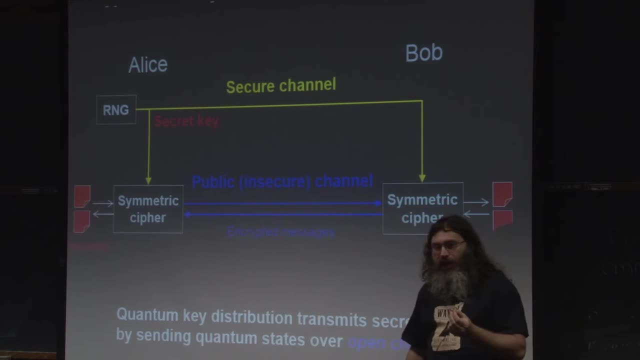 perfectly copied. But quantum cryptography bases the encoding of information on the quantum principles. It encodes single quantum states of photons and sends them over a public communication channel which can be subject to eavesdropping. But a single quantum state cannot be perfectly copied. 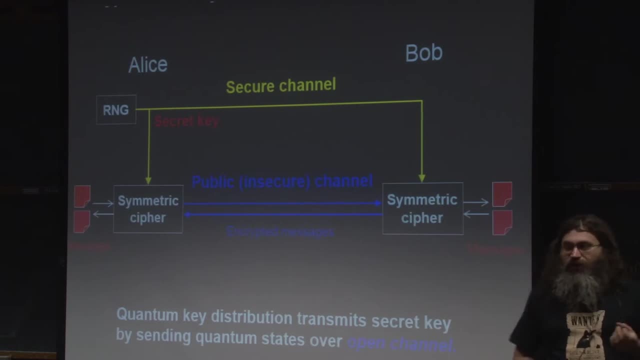 The physics does not allow that. If somebody tries to copy the quantum state, to measure the quantum state, part of the information is lost and this somebody will introduce errors in the communication which are then noticed by the two legitimate users. So, in essence, 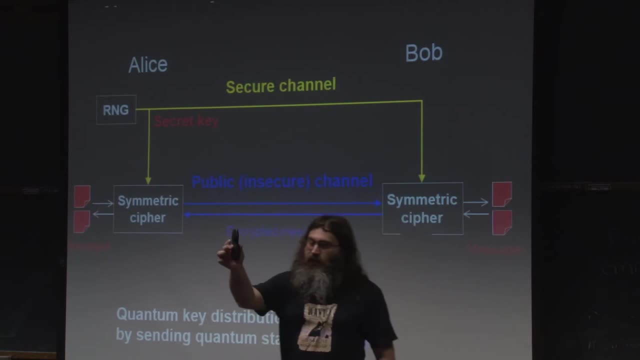 the quantum cryptography is based on the Heisenberg's Consistency Principle. If you have a particle and you measure the position of the particle, you know. here's my particle at this position. you know the position exactly, but at the same moment. 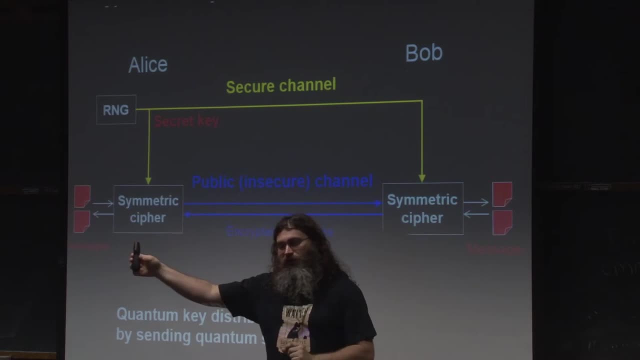 you lose information how fast the particle was moving, Or you can choose to measure how fast it was moving. you get the exact speed, but after that you have no idea what was the position. Such incompatible properties also exist for photons. This is the first time. 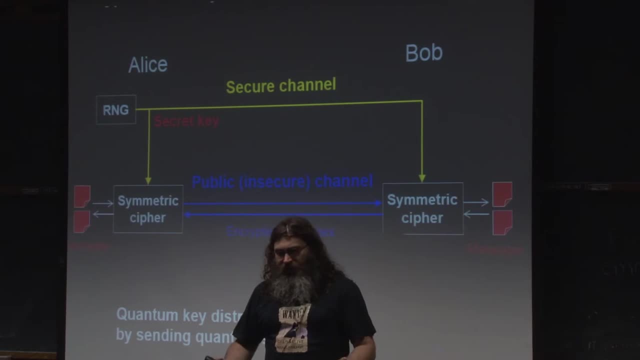 in the history of cryptography, in the millennia long history of cryptography, when we have a cryptographic algorithm whose security does not depend on assumptions of complexity or assumptions of difficulty, but it is based on the hard and cold laws of physics. Let's see how. 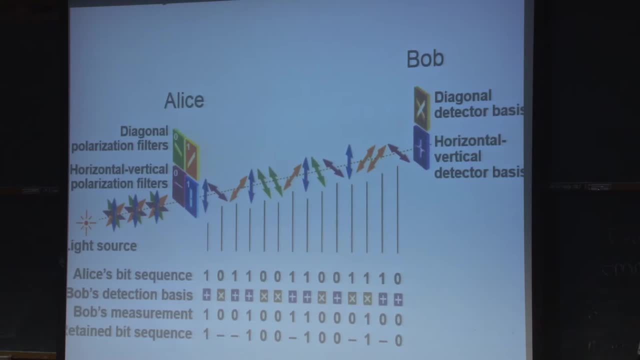 the sender, Alice, can distribute to the receiver, Bob, a secret cryptographic key using polarized photons. And, by the way, you can stop me and ask questions at any time. You are very welcome to do so. So if somebody, something is not clear, 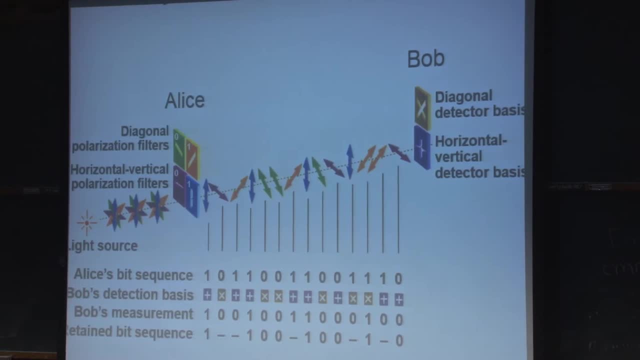 or you want me to slow down and explain something again. please do it. Alice, to send the random secret key. Alice sends to Bob a sequence of single photons. Alice randomly prepares the polarization on each photon In one of the four possible states. 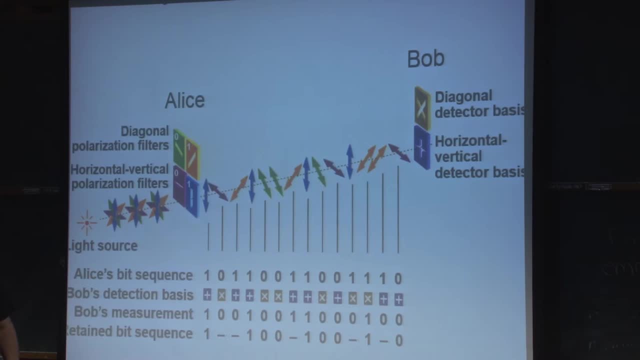 vertical, horizontal and one of the two diagonal polarizations. She chooses this polarization randomly for each individual photon. Bob tries to measure the polarization of the photon, each photon randomly, choosing between two incompatible measurements. Either Bob tries to measure whether the photon 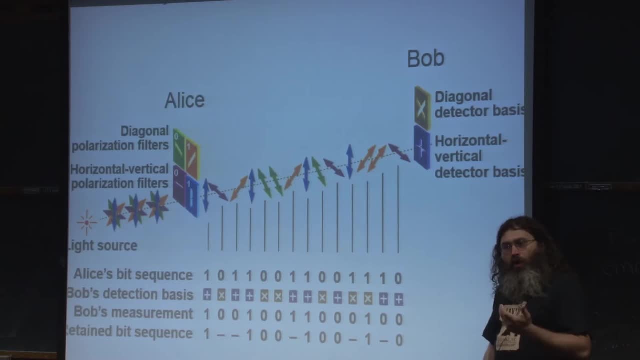 was horizontally or vertically polarized, or he tries to measure whether the photon was diagonally polarized and in which diagonal polarization. Those two measurements are incompatible If Bob measures for the vertical or horizontal polarization but the actual photon was encoded diagonally. 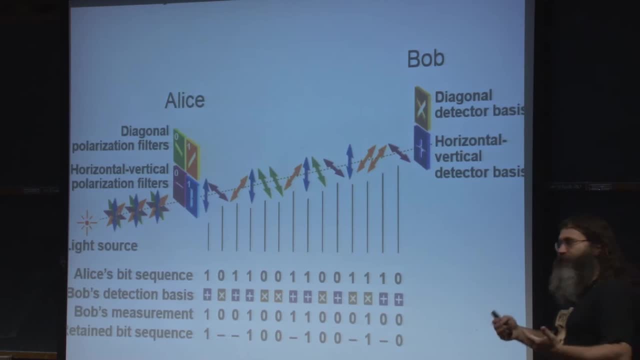 Bob just gets a random answer not correlated to the original polarization, But when Bob measures in the correct polarization. so if the photon was vertical or horizontal measurement basis, then he always measures the vertical polarization. So remember the choices are random. on Alice. 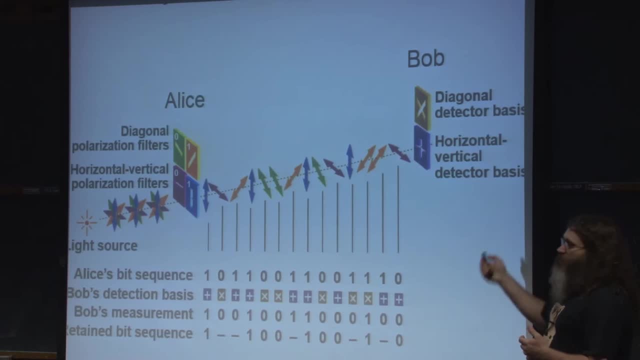 and random on Bob and those choices are independent between Alice and Bob. So each one chooses, makes the random choice individually. After a number of photons has been transmitted, Alice and Bob use a classical communication method. They tell publicly whether Bob and Alice. 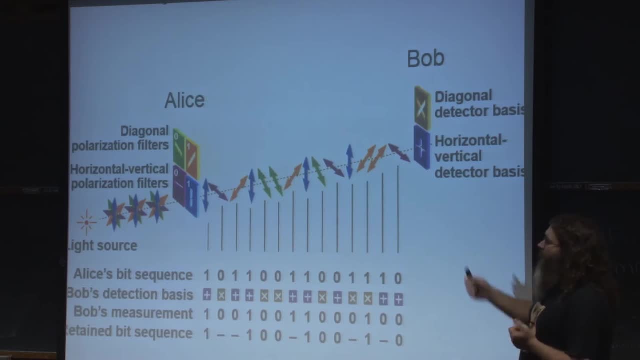 used this type of encoding or this type of encoding or that type of encoding, but not the bit value. So they only tell the basis- vertical, horizontal or diagonal- but not which bit value, not which of the two polarizations and not the result. 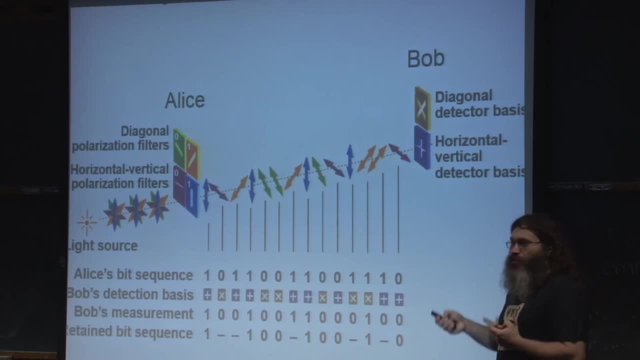 of Bob's measurement. In the half of the cases Bob will happen to have the same encoding. So say, Alice prepared a diagonal photon and Bob tried to measure it in a vertical, horizontal polarization- In this case, Alice and Bob. now 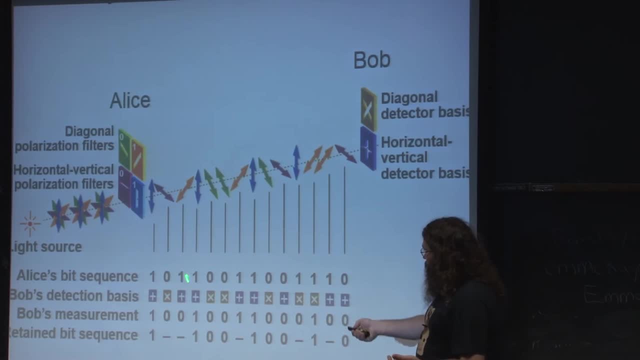 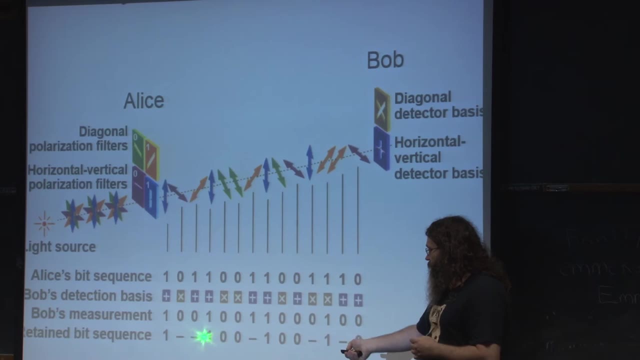 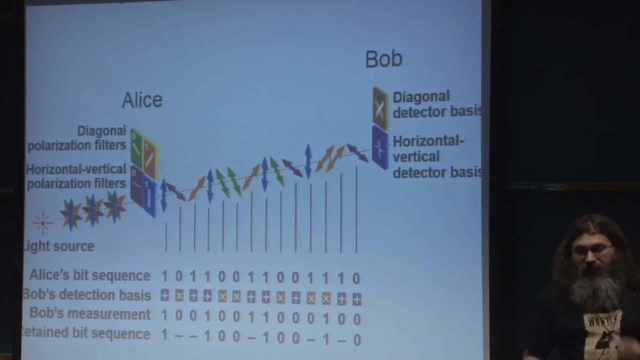 Bob's detection results were random and half of the time they were wrong. So in this case, for example, Bob measures a wrong bit value. Alice and Bob did not match. In the remaining half of the cases, Alice and Bob measured in the 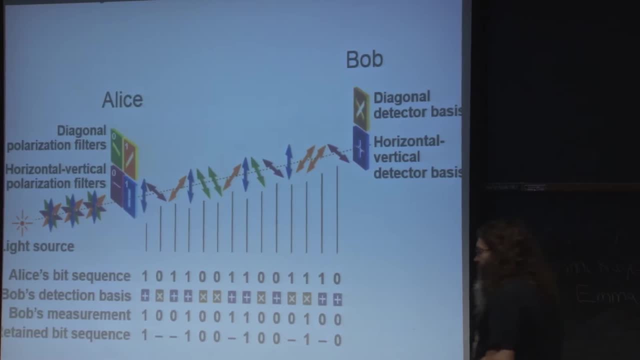 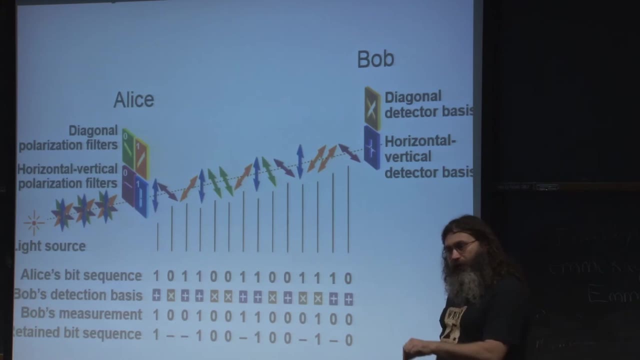 prepared and measured in the same polarization encoding And they bought. now that their bit value or the polarization states they used and measured were the same, Those bits form a horizontal polarization. So Alice and Bob measured the polarization of photons when they are being transmitted. 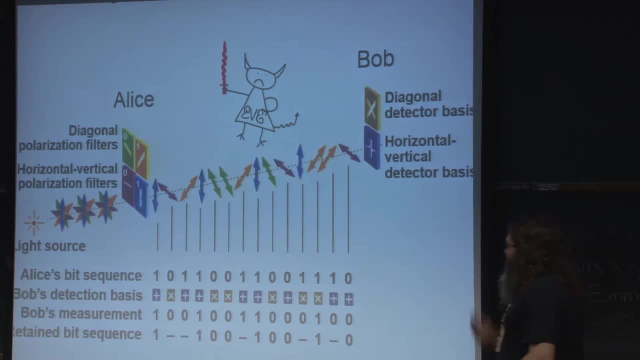 from Alice and Bob. At that time Alice and Bob don't announce yet the encoding and measurement of the photon. So Eve does not know in which polarization system the photon is encoded. She has to guess, And half the time she will guess. 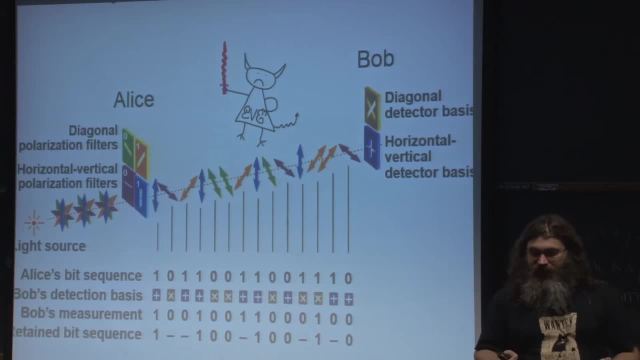 wrongly, She will guess that the photon is not in the same encoding as Alice And she will get random results. Bob says: sorry, I failed to detect the bit. Let's not use it. For Bob to use the bit Eve has. 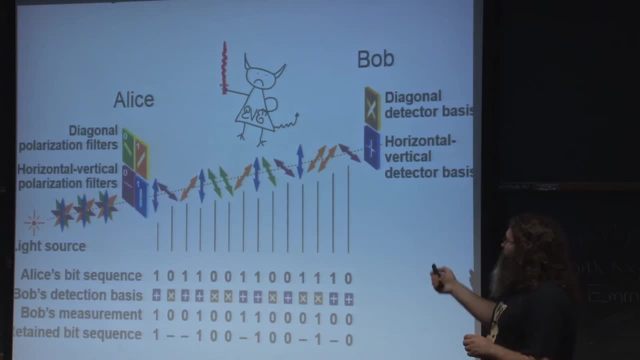 to regenerate according to her measurement result and send to Bob. And when Bob measures the photon in the sequence she gets the basis wrong. Dot introduces errors in this shared sequence. So Alice and Bob can compare a randomly chosen subset of this sequence. 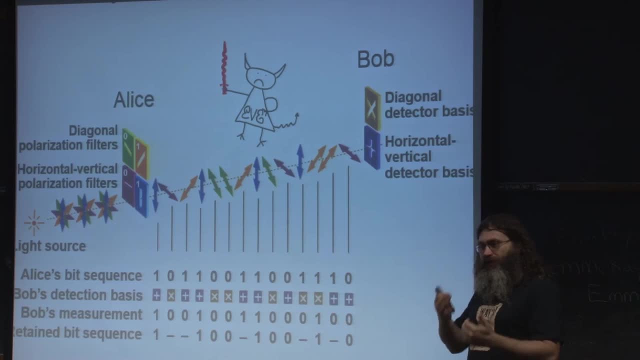 some part of it, randomly chosen part of the sequence, Then this signals to them that somebody might have tried to eavesdrop on the communication channel, And then they can discard the entire key and start over, So eavesdropping. 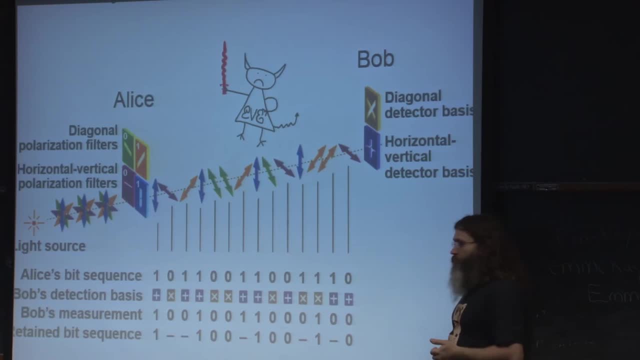 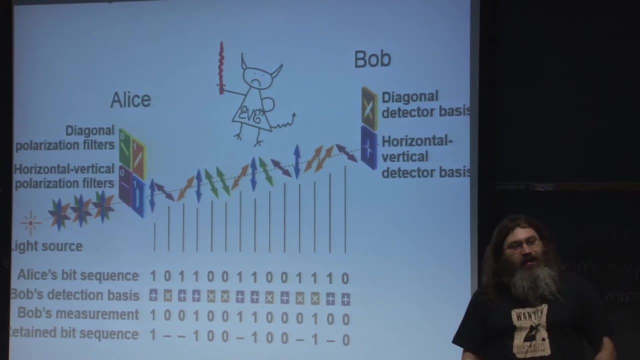 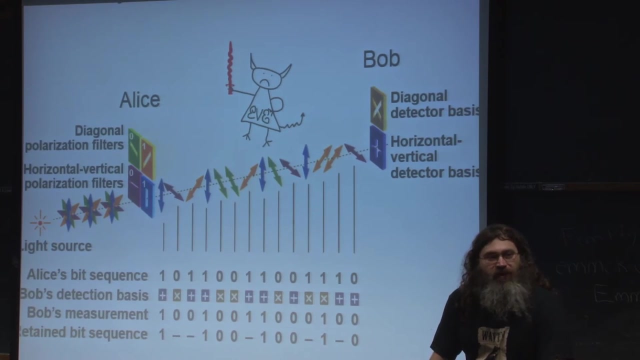 on this communication is, in theory, impossible, Any questions? Well, if everybody understands, the question is: if there is no eavesdropping, then will Alice's and Bob's bit sequence be identical? We mean those final sequences after they. 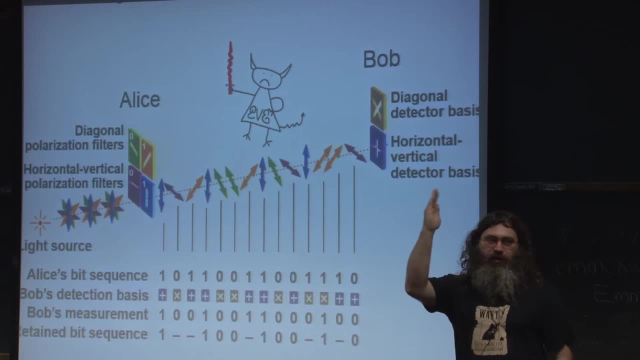 discard incompatible measurements. In theory, yes, In practice, even in the absence of eavesdropping, this bit sequence will contain a small fraction of errors, small number of errors, And you can still make a secret key out of it by running. 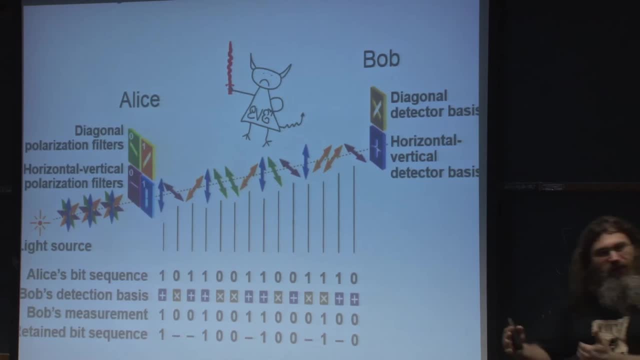 an error correction algorithm And if you have not too many errors, you can still show a number above 11% errors. Above that, you cannot get any secure key out of it, But if you have less than 11% errors, 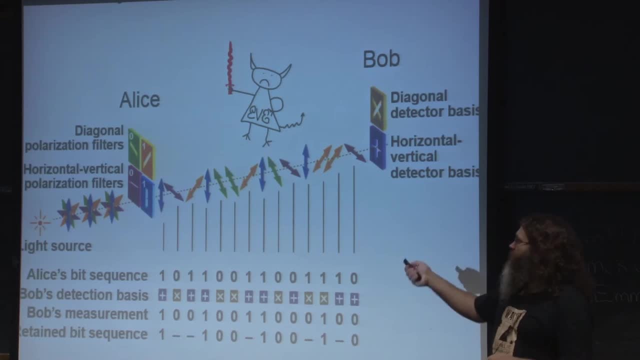 then a certain type of error correction and compression of the key will allow you to get a secret key. So we know our threshold percentage above which we have to discard the key and below which we can try to extract a secret key. That is a practice. 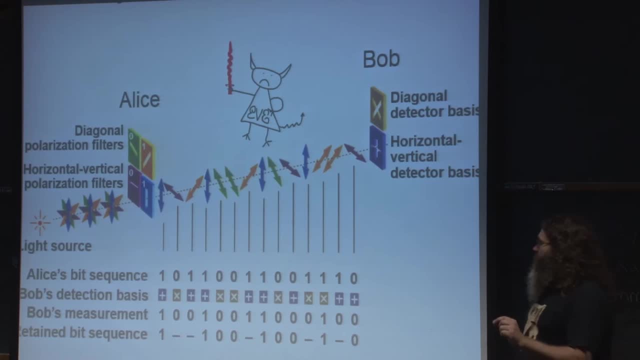 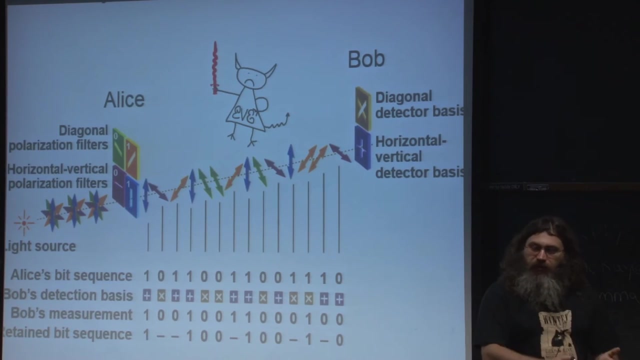 Of course it's a very good issue. You can never get identical sequences, More questions. Of course they need to verify this. If they want to use the key, they have to use an identical key, Otherwise the decryption will fail. 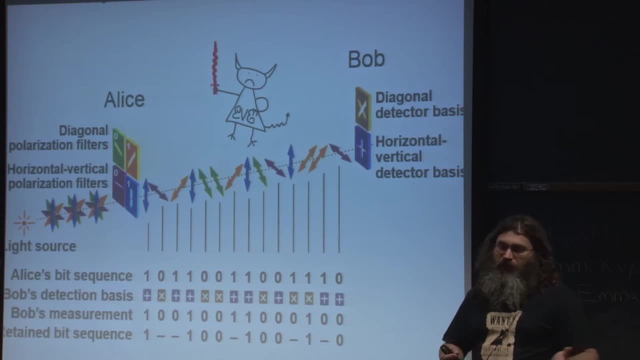 In principle, they can do just that. They can try to use the key for encryption and if the decryption fails, they can use the key for encryption. If the key fails, they can use the key for encryption. So what they have. 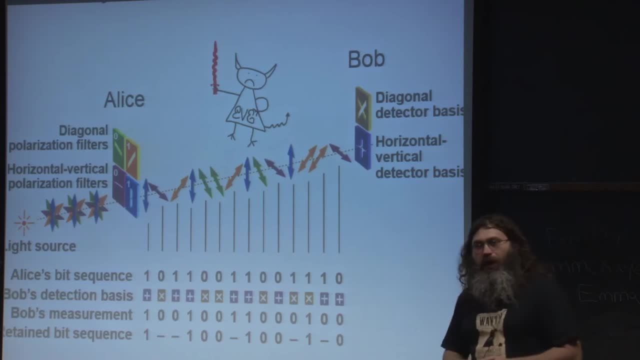 to do is to use the key for encryption. In the process of decryption, the key is discarded from the key. So there is the identity check procedure. It's in the practical protocol. Is this clear? More questions? Yes, So. 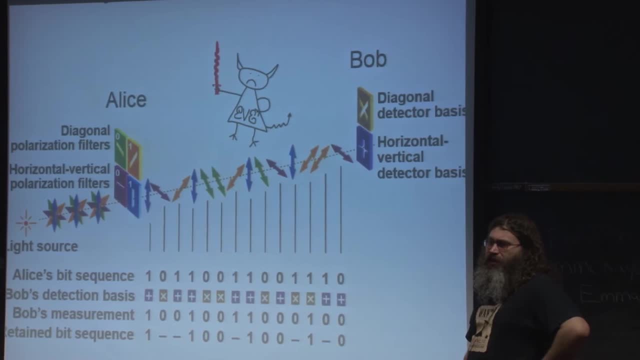 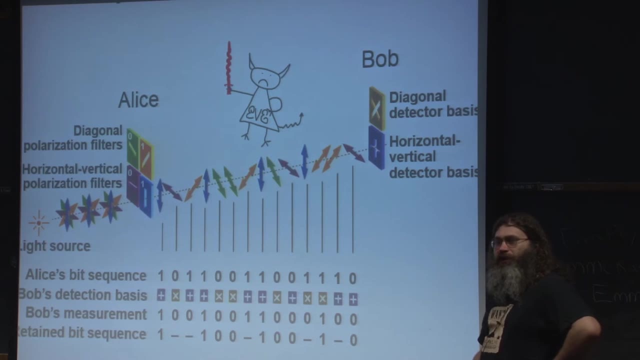 what are the things that you have to do to decrypt the key for encryption And then how can you decrypt the key for encryption? So what do you do in with all those states at once, as in as to one state? so if is allowed to do anything allowed, 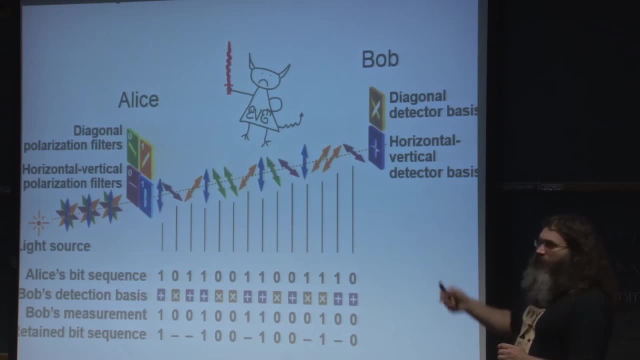 by the laws of quantum mechanics. so, in fact, the simple explanation i have given you, if you look at the details of the security proof, this is not what is used. this is just, uh, to give a feeling why this is secure. yeah, so sorry. the answer to the question first. i don't know it. you can ask. 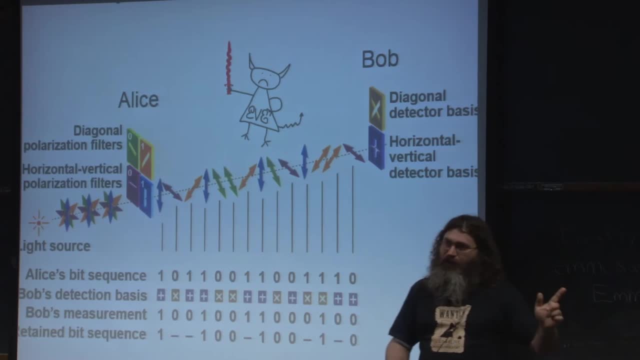 norbert lutkin house at the aqc. he works with the security proofs he might be provide, provide you a better answer. and second, the answer will be much more complicated than i can explain today. but there is an answer and it's a strict security derivation. just logic it's. it's not an 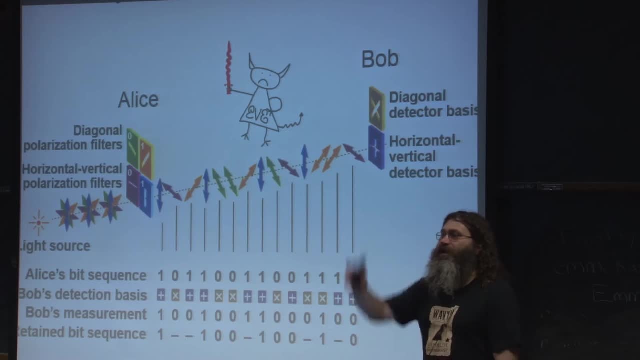 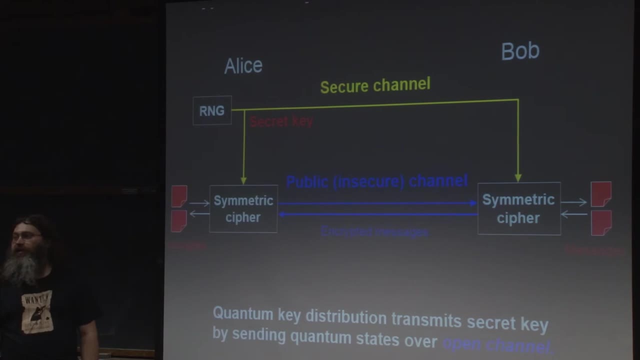 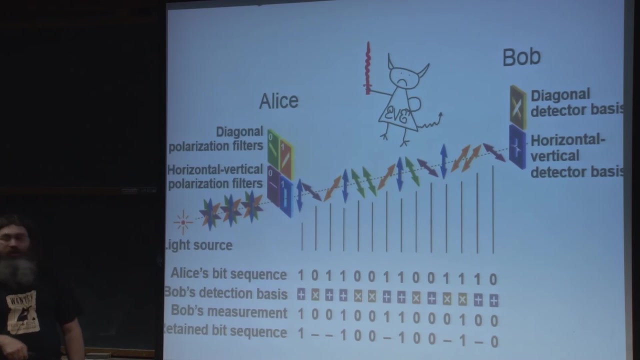 assumption: yes, please, okay. so the question is about the classical encryption. how large does the key have to be in order to encrypt information, you right? uh, oh well. or, or did you ask a different question: how many bits of information do we have to discard? uh, so you lose half the bits during the comparing of the basis. this is inevitable. 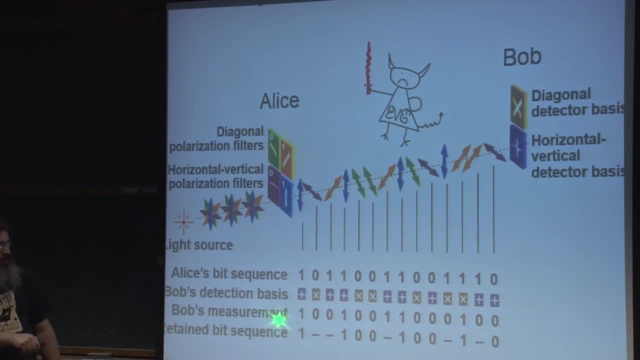 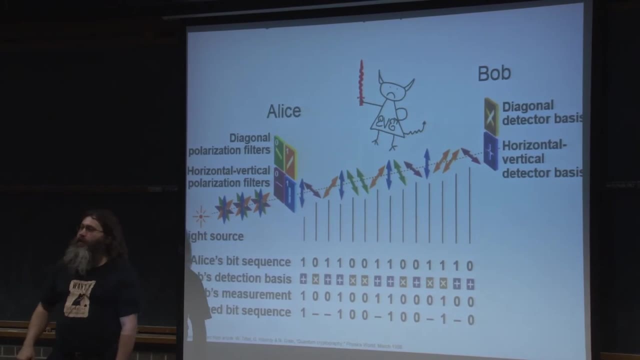 and then the check if the key is sufficiently large, like we have only, uh, nine bits on the screen, but realistic keys are millions of bits and in a million bits you do. you use only a small fraction of the key to check for eavesdropping, so most of it you get out if you have a large. 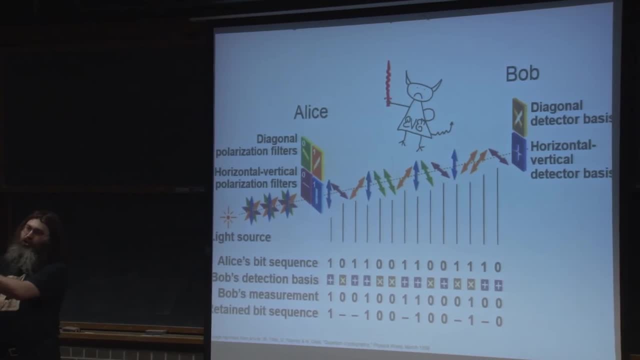 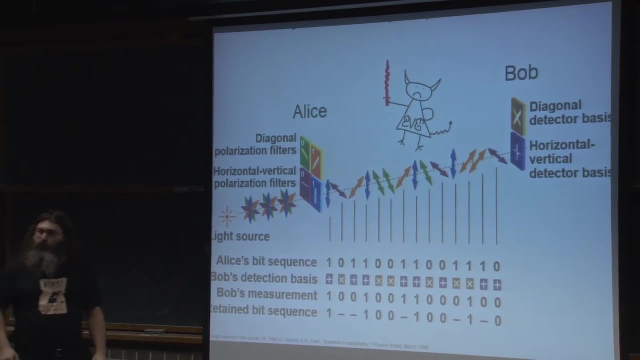 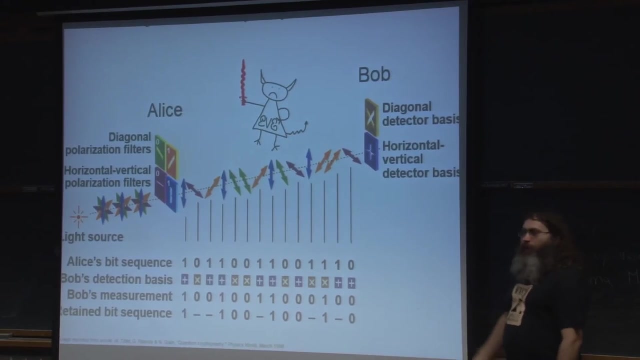 key, then you can show that checking only a small portion of it already gives you a statistically sound ans第二個, the rest of the key. so you don't lose much if you have a lot of key to begin with. well, i believe we should on and go to implementations of quantum cryptography So you can use polarization to actually do. 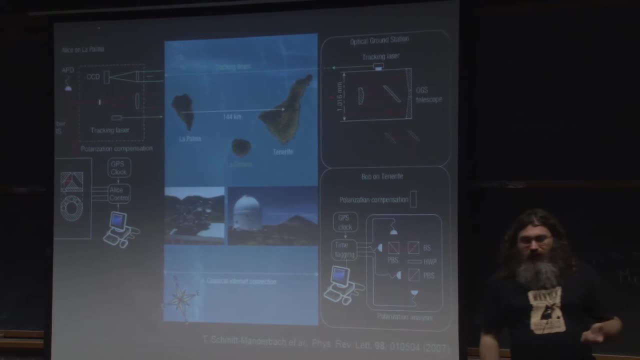 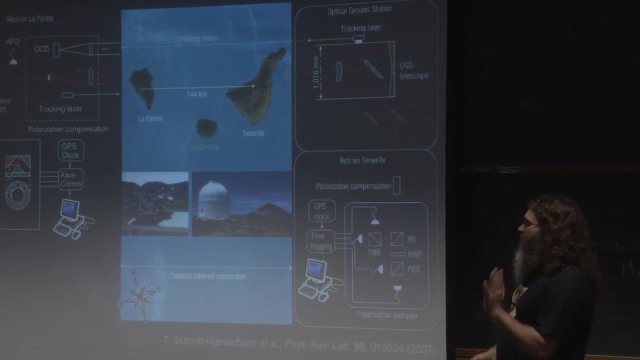 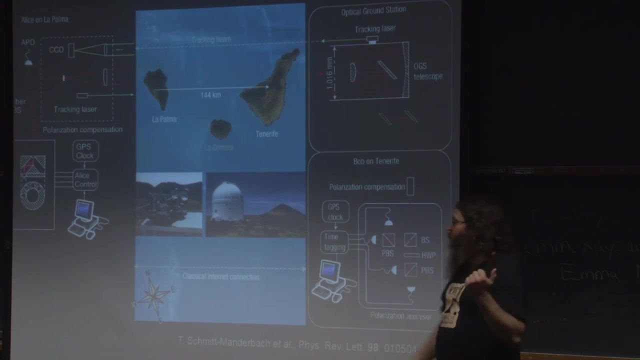 communication. This: if you are sending and receiving your quantum states over a free space, over air, air holds polarization very well. If you polarize the photon and send it over to 100 kilometers, what is received is the same polarization. So this is the longest. 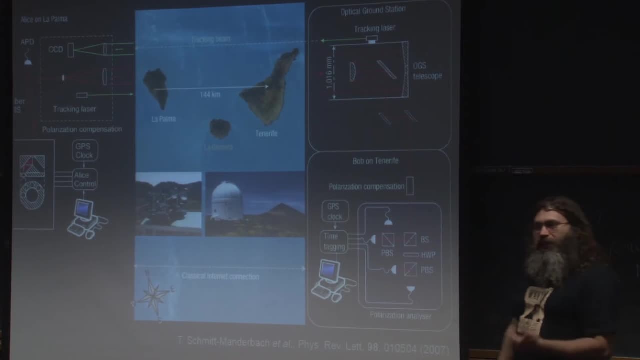 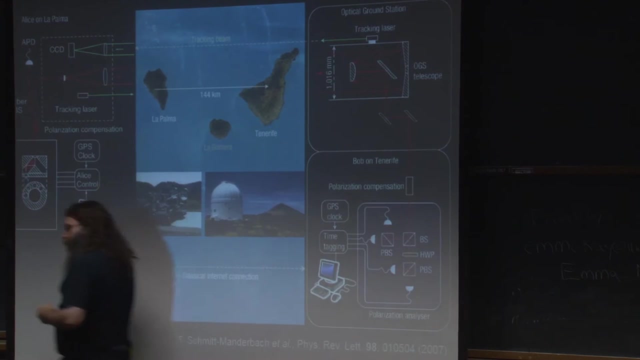 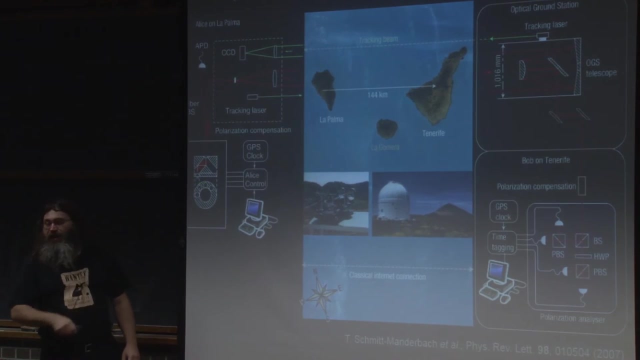 quantum communication experiment which was demonstrated to date 144 kilometers between the two Canary Islands of La Palma and Tenerife. In the sender station to form, to make the four polarization states, Alice is using four laser diets. So if you take a semiconductor, 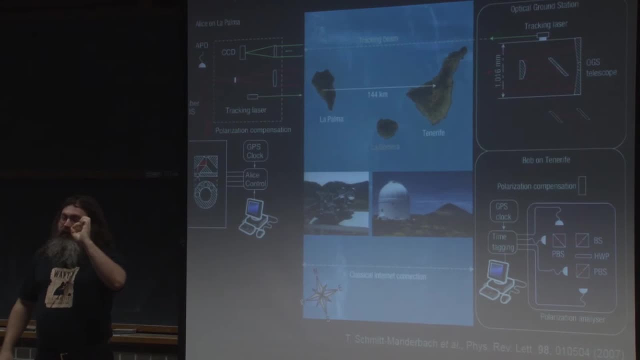 laser diet like the one in your CD player. the dot semiconductor laser diet is emitting a highly linear polarization, So you can get your four polarization states, but simply rotating the guide, the diet at the angle, And there are four laser diets activated at random their outputs, and they are rotated each to vertical and diagonal. 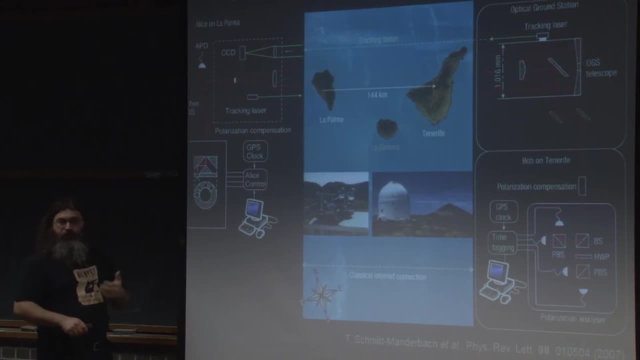 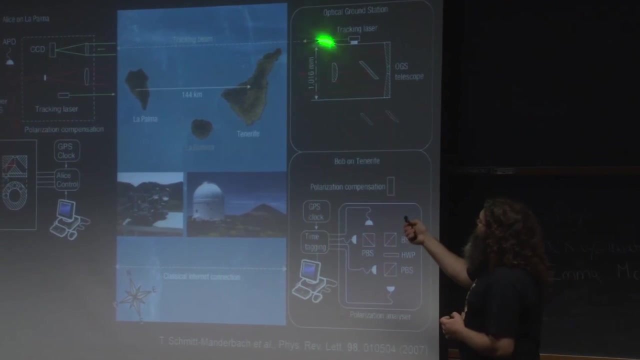 and 40,, 90 degrees, 45 degrees comparing to the axis of the laser crystal, And then the signals are combined and sent from a telescope over to the other island. At the receiver station, the receiving telescope collects the light. 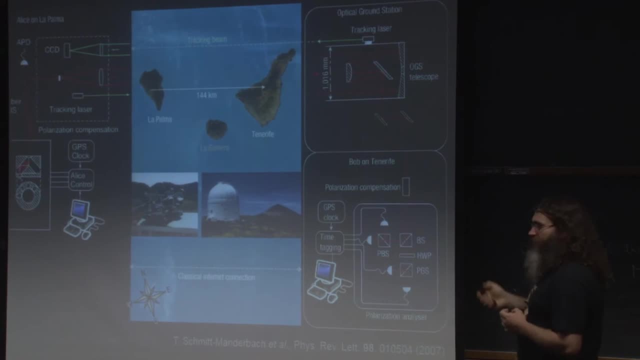 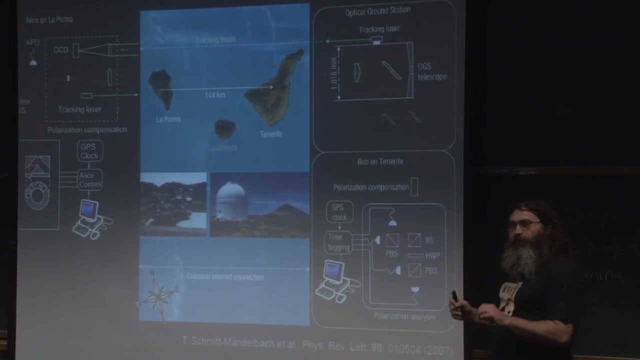 So we have a there is a polarizing beam splitter. so this beam splitter splits the photons vertically polarized into one path and horizontally polarized in another path, and two single photon detectors looking for photons. in the other arm the polarization is rotated 45 degrees. 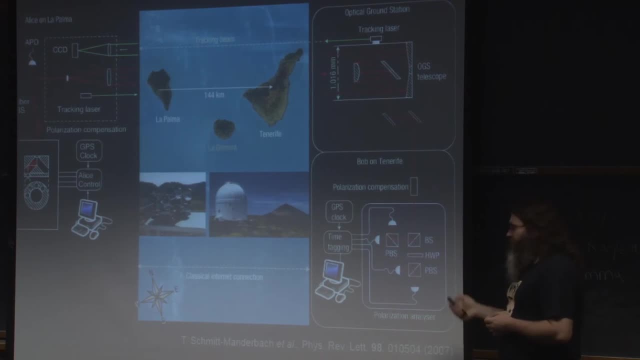 and again. there is a polarizing beam splitter and two detectors. but because it is rotated, this arm is looking for two diagonal polarizations and this scheme works very well and you can transmit and do the key distribution. when you want to do it at such a long distance you have to use a big telescope. 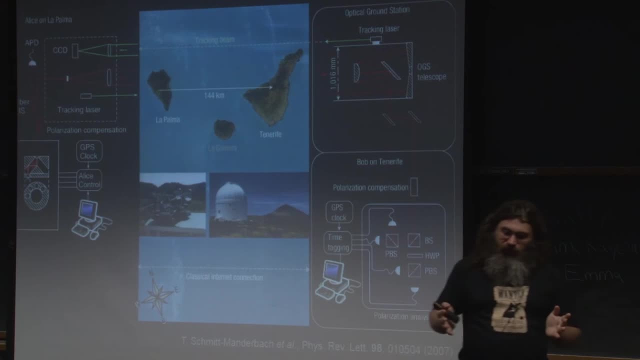 if you don't need 100 kilometers, you can do it with small equipment. some several demonstrations have been made with over tens of kilometers where you can use essentially a desktop equipment, and one of those demonstrations happened here in waterloo between the buildings of the university. another research group had this demonstration several years ago. 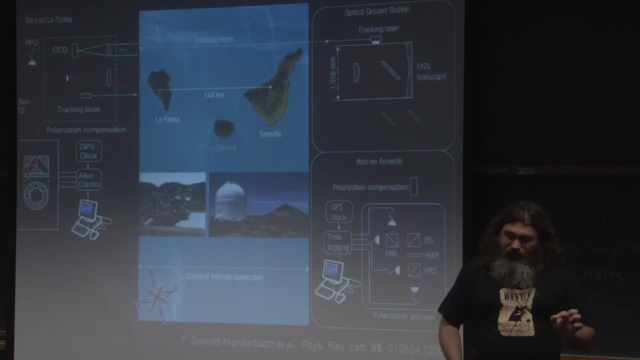 this is over free space. this is one way to transmit. another type of communication channel is an optical fiber, the standard installed optical fiber which we have all around in the installed optical networks. and if you want to transmit over an optical fiber then you have to use a different. 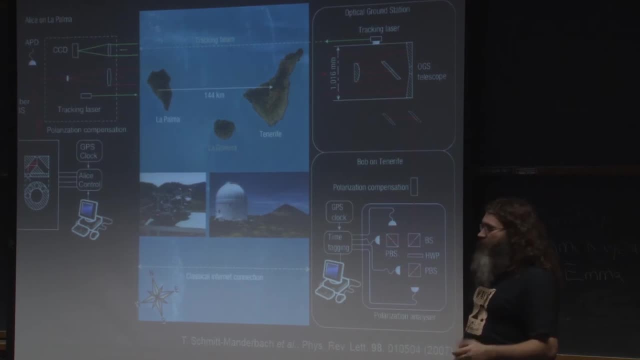 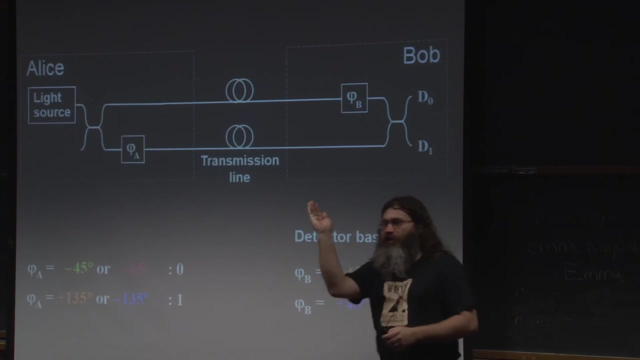 encoding, or rather it's easier to use a different encoding fiber does not transmit polarization very well. if you transmit polarization in the fiber, the polarization will rotate and become elliptical, generally speaking, and this transformation will change when the temperature of the fiber changes or the conditions of the fiber change, which happens all the time. 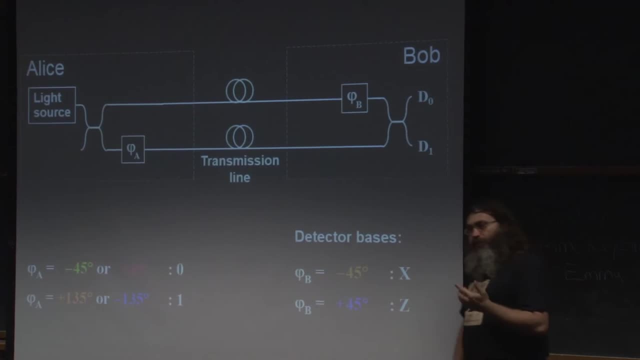 so a more convenient way to use is to use face encoding in fiber. in essence, a fiber optic encoding scheme is a mach center interferometer, the the consisting of two arms. the alice's laser is split into two arms and then combined into the two arms in bob on a 50: 50 beam splitter. so in this interferometer we will have 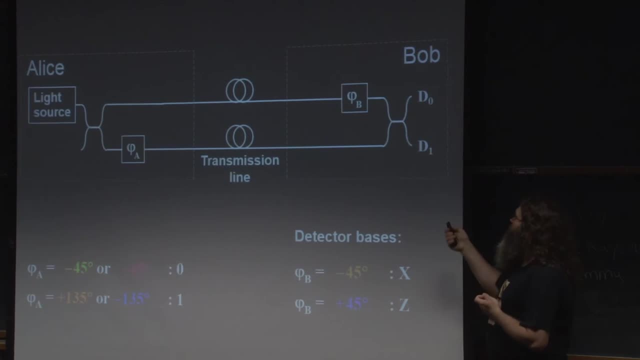 interference at this beam splitter. and behind the two outputs of the beam splitter there are two single photon detectors. which detector the photons will go to depends on the combination of phase settings. so alice has a phase shifter and bob has a phase shifter. it's the uh some, or rather this: 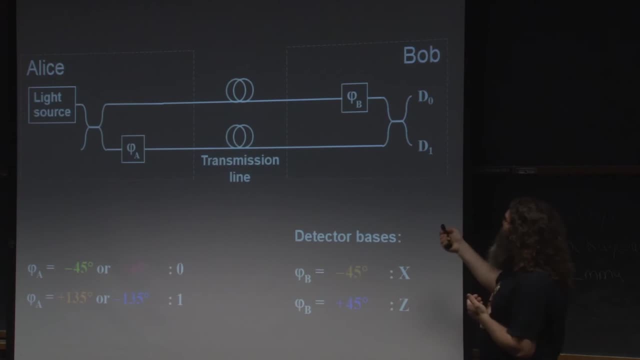 phase minus dot, phase is. dot determines which output the photons will go to, and the encoding is done the same way as with polarization, except that instead of preparing polarizations, alice makes one of the four possible phase shifts using this phase shifter. so essentially a small delay of a delay. 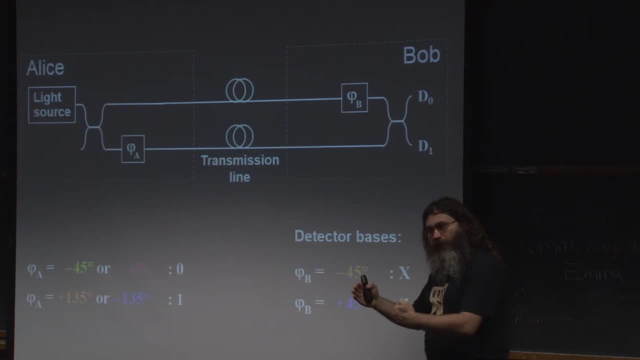 to the transmitted photon corresponding to a fraction of the wavelength of light. we call it a phase shifter. in fact it's a delay line which works on a very, very small scale- a fraction of wavelength- and bob makes one of the two possible phase shifts using his phase. 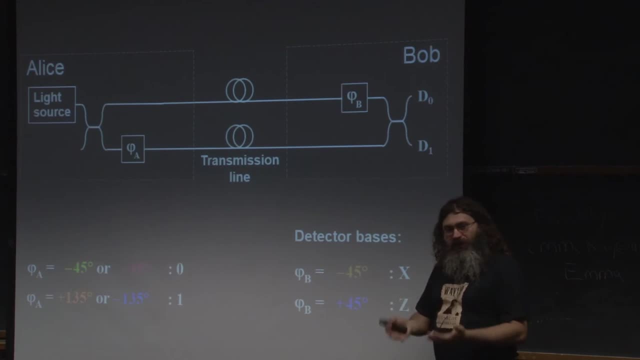 shifter and alice's encoding corresponds to the four polarization states and bob's phase shift corresponds to the choice of the measurement basis. and then they control whether they have good interference, which allows bob to read the same beat as here is prepared, or the result of bob is random. the functioning of the scheme is exactly the same as with polarization, except that 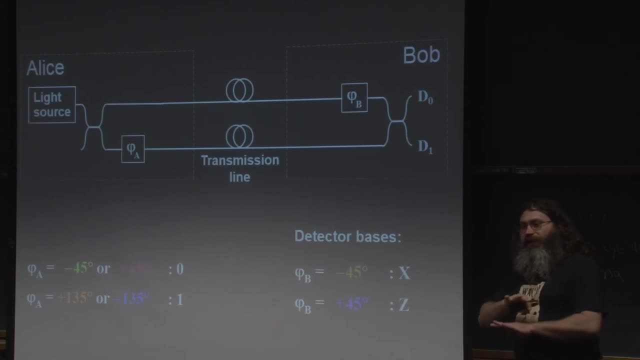 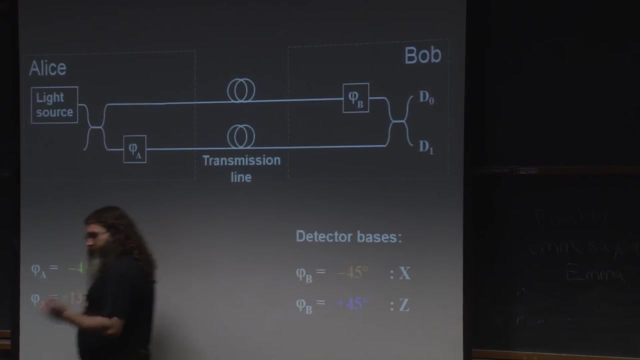 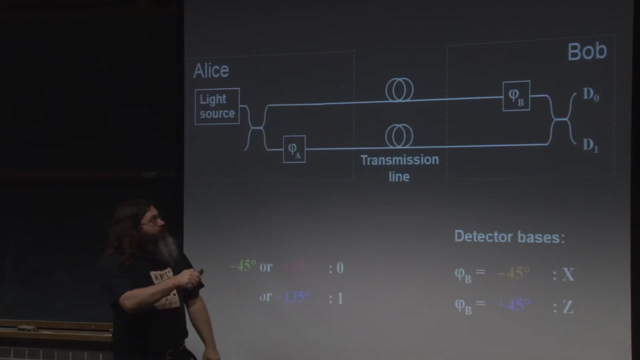 instead of polarizations, we have two phase shifts and two phase shifts here. the rest is identical. you can build a scheme and there are companies selling this scheme, for example. yes, and one other small detail in this scheme: you will have to run a long, two long fibers, which is 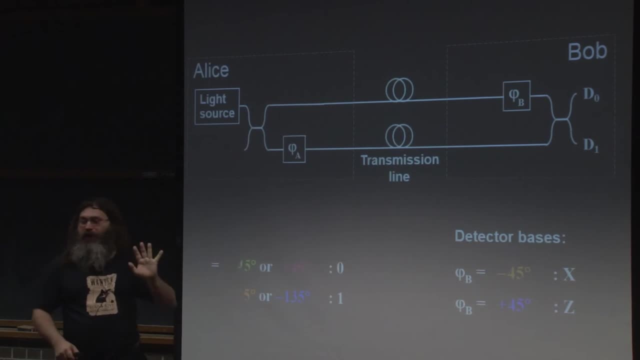 impractical, like, first, it's two fibers and, second, this interferometer will be very, very unstable because two fibers are in separate conditions. so this the other thing you want to do: you want to multiply the pulses. time multiplies the pulses into a single transmission line and then demultiplies them. 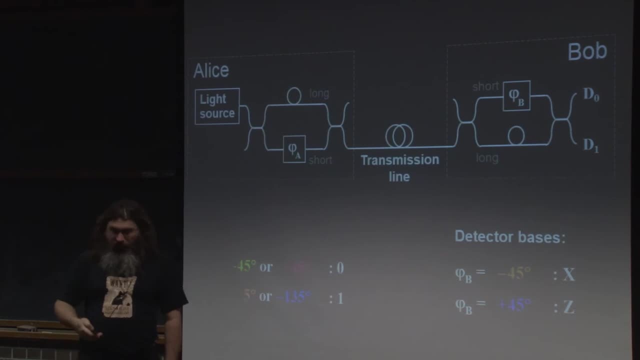 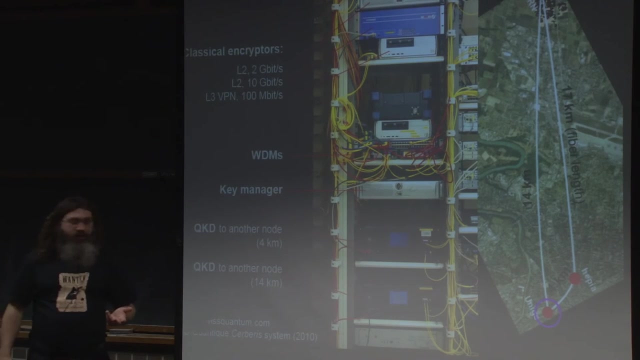 so this is done and you can use standard communication fiber there and you can go and buy this system from one of the companies, for example from id id quantica, swiss company, and this is how it would look, installed in your server room, if you have enough. 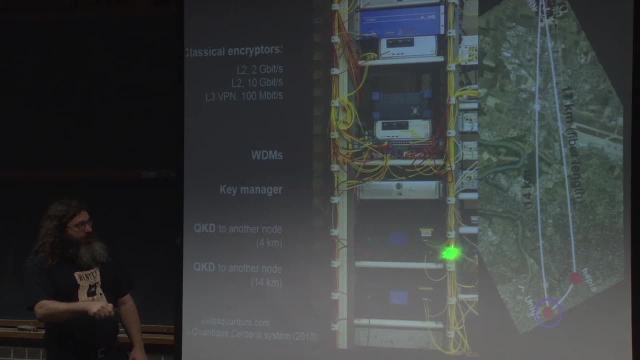 money to buy this equipment. you will have quantum communication boxes which produce secret keys with two other remote nodes. so this is the picture of this in the installation in switzerland, and those boxes each communicate with one on other remote node and then they produce keys and they pass those keys to a bunch of classical 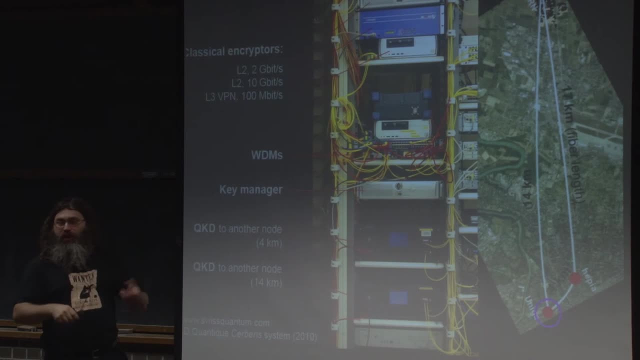 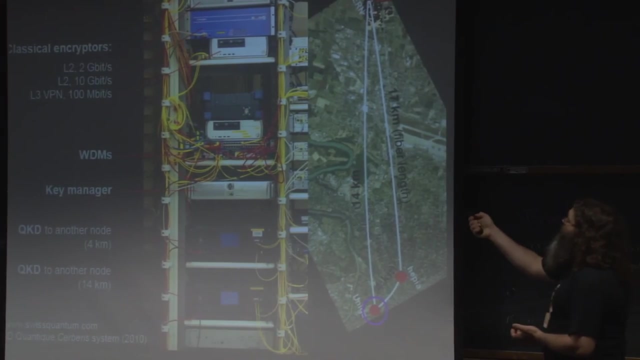 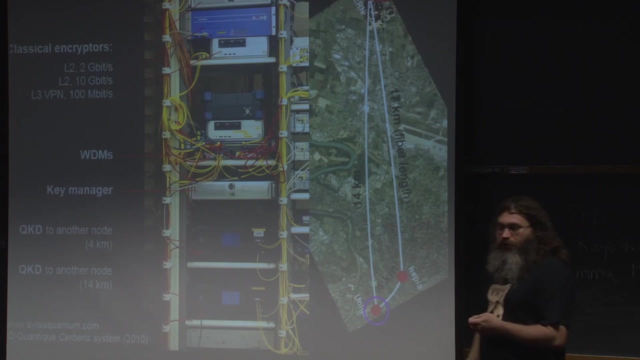 encryption equipment. in this classical encryption equipment your actual encryption of information occurs. so this node encrypts all fiber optic communication between itself and other nodes, and this demonstration in switzerland formed a small network. so you have like a triangle between three links, two at the university and another is at cern, and they wanted to encode uh results. 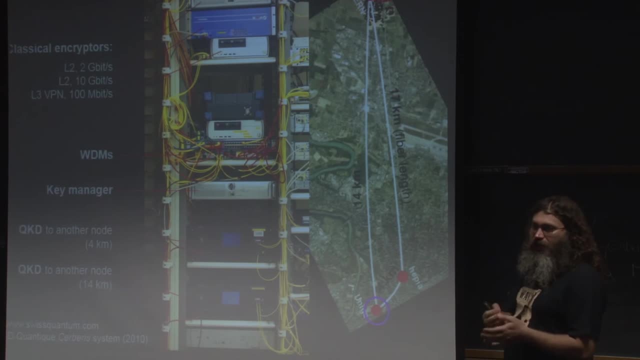 from the large hadron collider. but the large hadron collider didn't run at the time. it was delayed, so they had to use a box to simulate traffic. but it worked very well. so you can make a network using standard optical fiber and if one of the network patches fail, you you still have. redundant patches so you can distribute the key between the nodes. the distance- communication distance over fiber is in or over free space- is limited because when you send a photon you have to begin with a single photon and it gets lost in the communication channel in practice, which this means bob starts to receive less and less photons the longer your communication channel is. 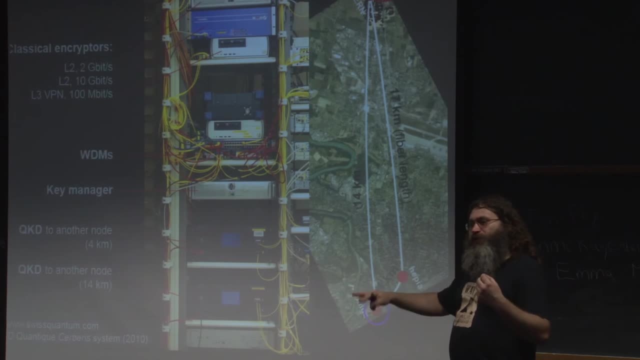 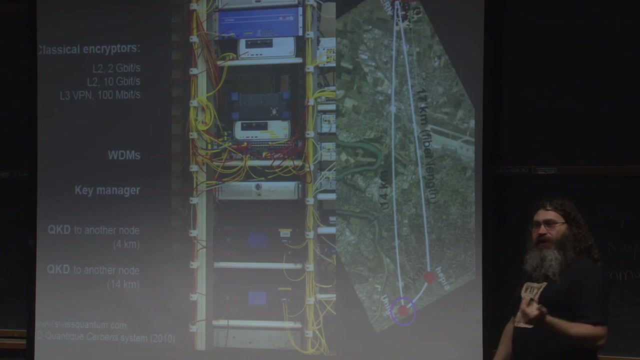 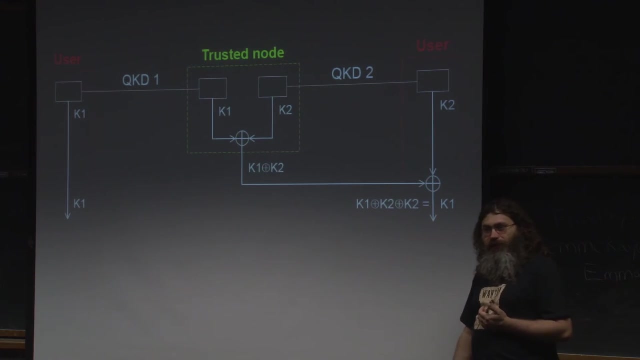 so key generation rate drops and eventually it becomes so low you can no longer use this channel in practice. so the single leg communication distance is limited in practice by one, two hundred kilometers. how to increase the communication distance to longer distances? you can chain the links. you can have one qkd link generating a pair of keys, and you can have another link, generating its own pair of keys. and it depends on how much is used by the internet link does not go much brighter than one這個 linkzth gradually. so black, black and orange dimensional right now again black, black and orange. you can decide between three these instead of two, that's. a single local forสd 0. this is like you can decide specifically if you want to account if this proxy only Eb- and i see it doesn't ¡öhh- is dollar or so a trajectory from here. this is what i'd exhausted, only at the edge. our 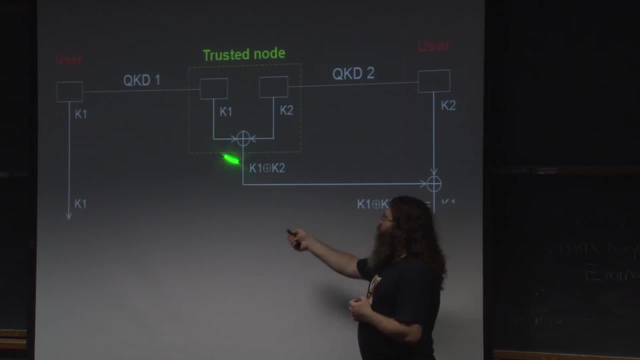 of keys and then, if you trust the node, this node, the node can encode one key with the other using bitwise addition, addition modular to the xor operation. so in essence, it one time pads one key using the other and this node publicly announces the result of this addition. so in essence this: 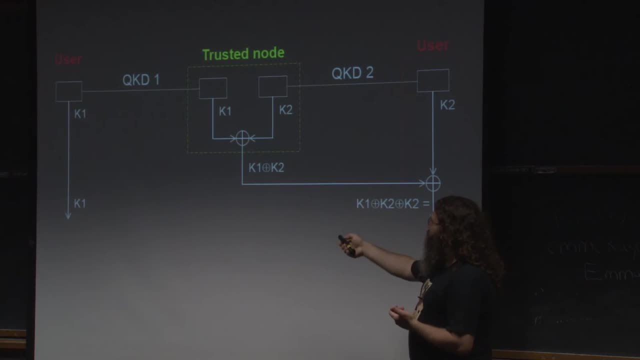 is a one-time path, an unbreakable cipher. when you use, in essence use one of the keys to encrypt the other and publicly announce the result, then the other node can use her copy of the key two to decrypt key one by again doing another bitwise addition and get the original copy of key one. 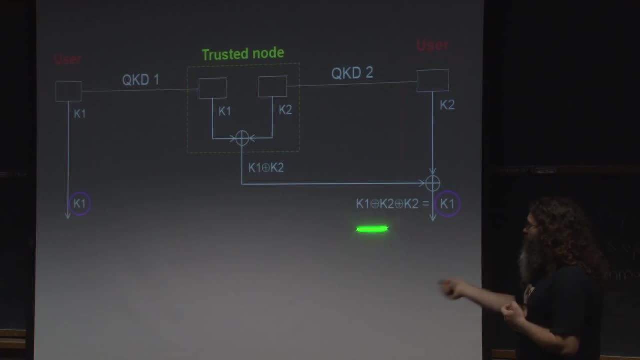 and then the two remote nodes share a copy of the key, even though they don't have a copy of the key, even though they don't have a copy of the key, even though they don't have a direct link, they have only, they are only on a chain of link between trusted nodes. 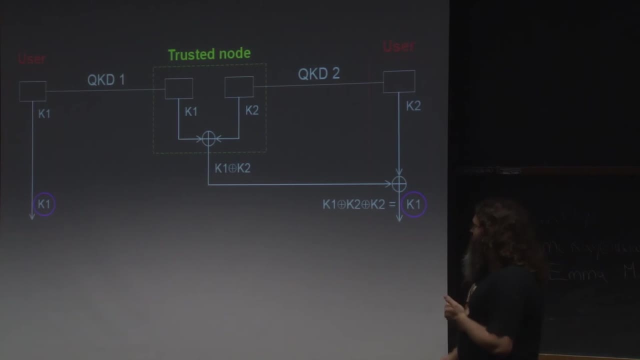 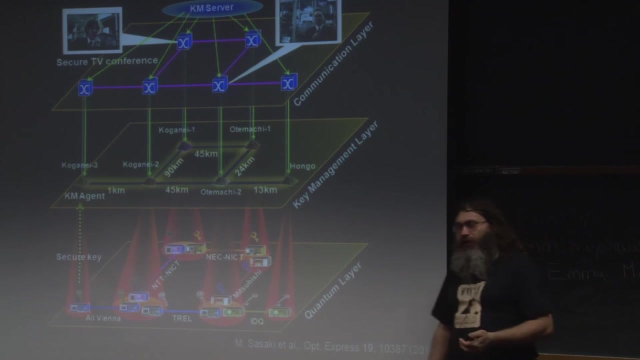 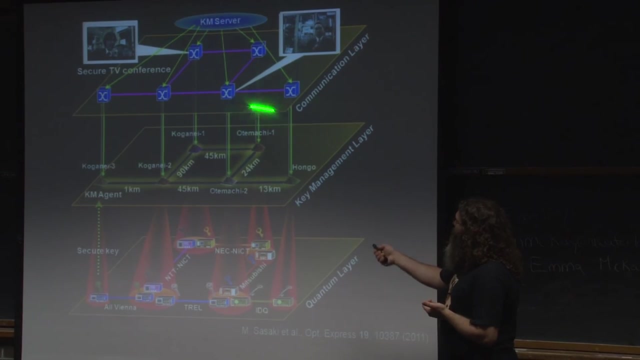 you can chain more than one node in such way and you can make a very large network this way. so, for example, this is a demonstration of a quantum key distribution network in the large, larger tokyo area, and you see that in this demonstration there were one, two, three, four, five. 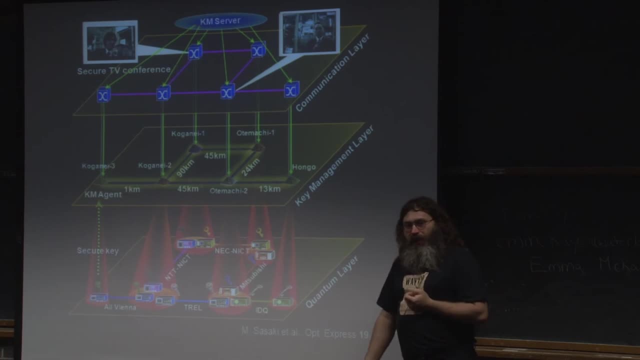 six nodes and six links between them, and there were many combinations of users when the users did not have the a direct communication between them but could have to go through intermediate nodes. so in this demonstration the qkd systems generated a bitwise pair of skis between the nodes, so each 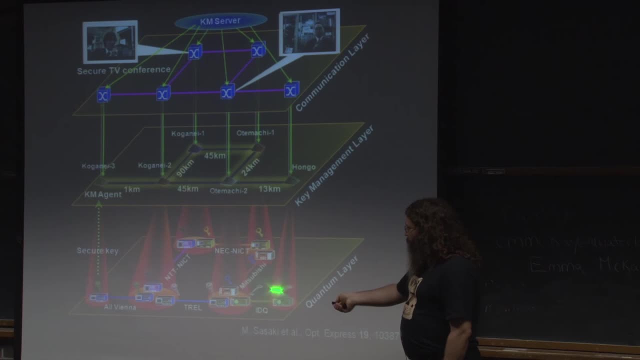 link generated its own pair of keys. the keys were stored at each node, accumulated in each node and when a pair of users not having a direct link between them wanted to communicate securely- say they wanted to encrypt a video conference call between them using quantum key distribution network. 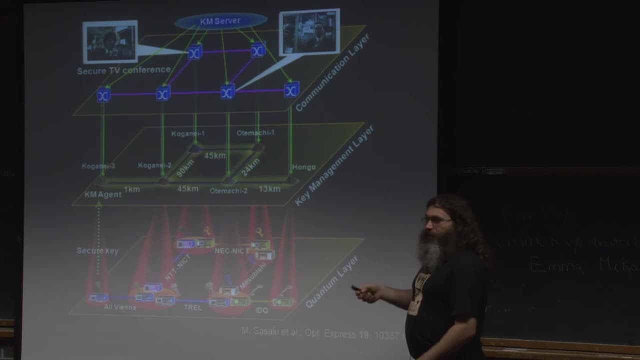 time part. they sent a request to the network software and the network software found a patch between the nodes to do this bitwise encryption and generate the key. give the secret key to the two end nodes. this works pretty much like internet. the software finds its way to root the key and if one of the links fails, it has another patch through the network to generate your key. it's open source, by the way, and such network demonstrations have been so done several times. so you can do it with the current technology over a metropolitan area or an area of a small country. 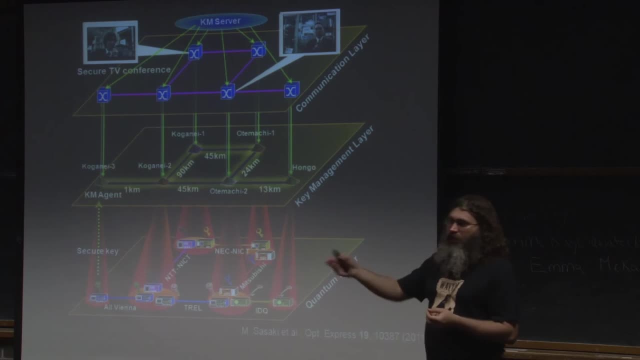 so say, if you wanted a link between waterloo and ottawa, we will just chain six or seven qkd systems through knots and we will have a secure link, as long as any of the nodes are secure. how to increase this communication to a global scale? it's pretty difficult to chain nodes when you go over the oceans. 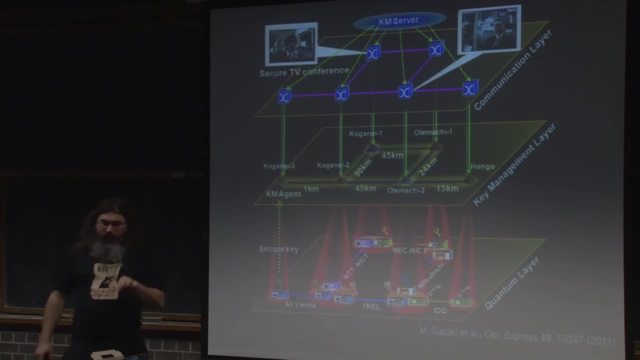 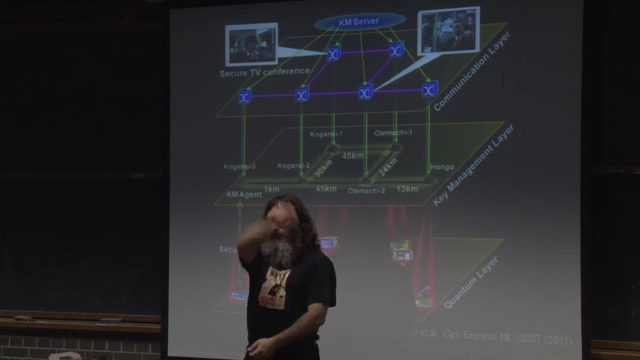 so you just need very many of them. so another alternative idea is to use a satellite and make the satellite a trusted node. so you have the globe and you let the satellite orbit your globe in a polar orbit and as the globe rotates underneath, your satellite will be visible twice a day from any point in the. 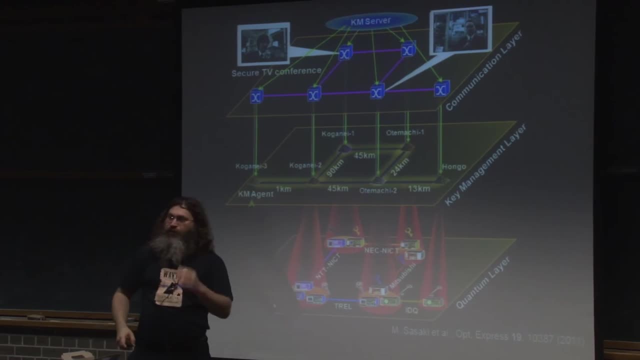 globe. so you can use a single satellite, do communications between one ground station and the satellite and then the satellite fries, flies to the other side of the globe and you can do communication between another ground station and the satellite and, using the satellite as the trusted note, you can establish the keys between two separate. 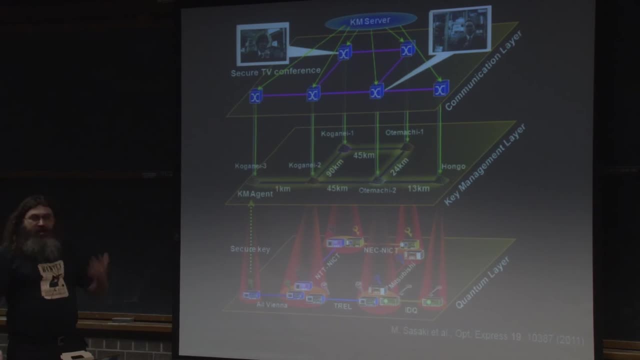 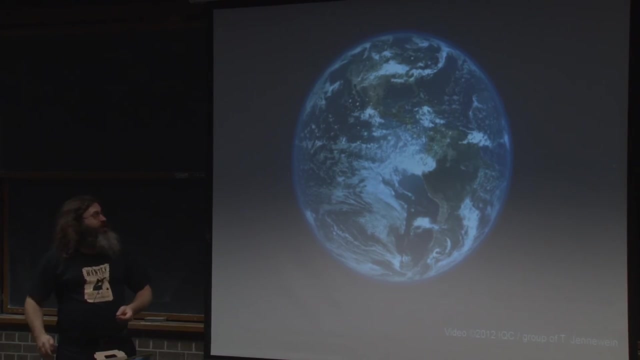 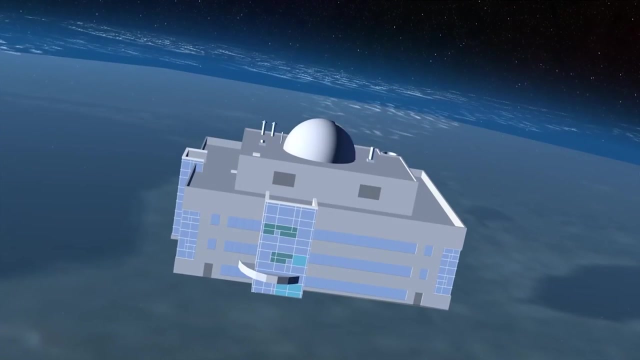 points on the globe, any pair of points on the globe. this is another thing that the University of Waterloo researches. we have the idea to launch the Canadian quantum satellite, and this is the video showing how this would work. so here you see the rack, one building, and we do actually have a small telescope dome on. 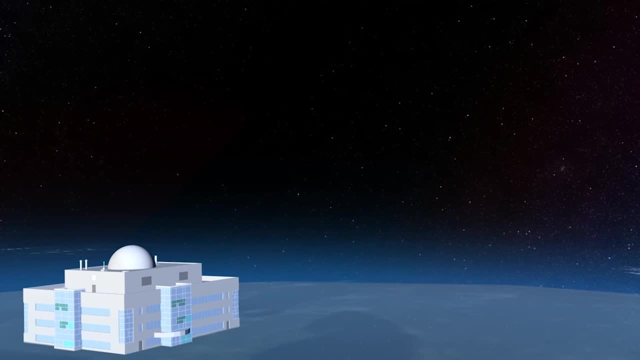 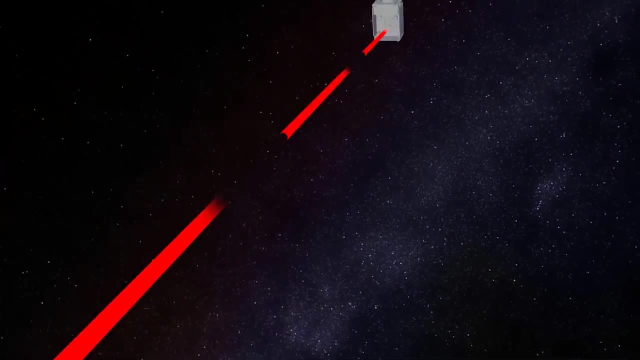 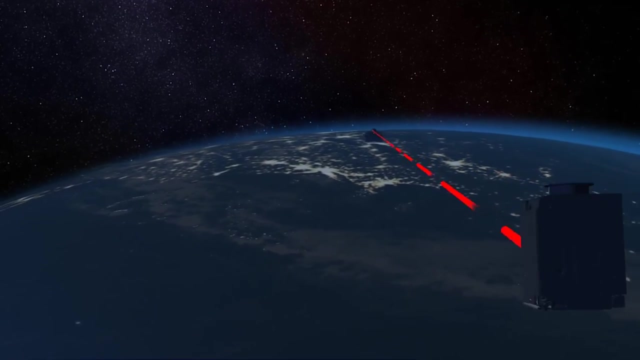 the top of this building used for quantum communication and he caps the Canadian quantum satellite- not launch it yet, but we hope it will. the satellite becomes visible and does the key distribution between the rack one building and the satellite. the visibility window is just a couple minutes, but it's enough to establish a good 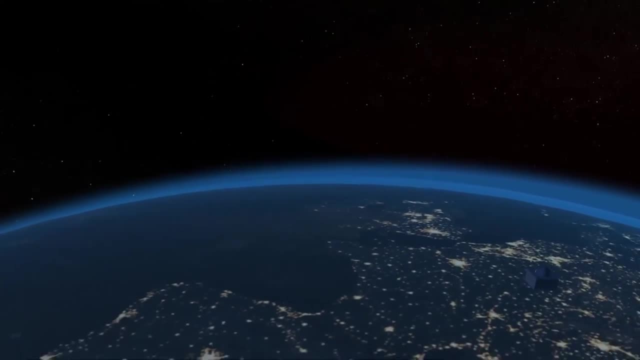 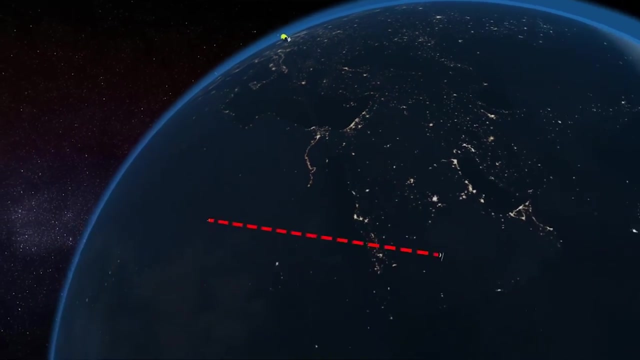 language between the satellite and the satellite. the visibility window is just a couple minutes, but it's enough to establish a good language of key. 40 minutes later, the satellite flies over Tokyo. is the Tokyo or some other part of the globe? no, this is Vienna, I think, and then Australia, and very 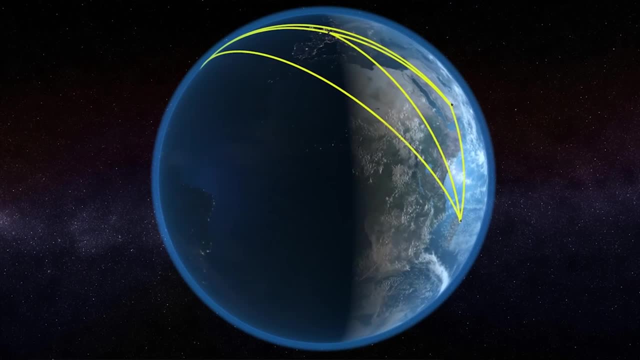 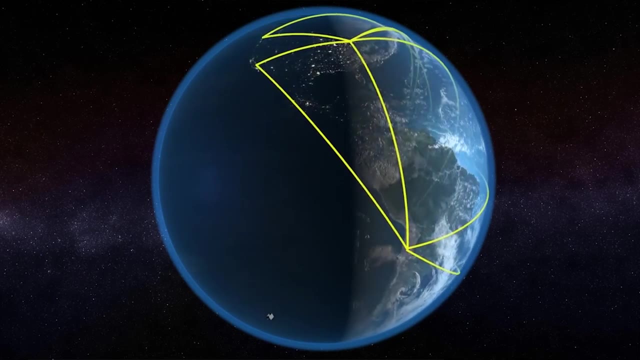 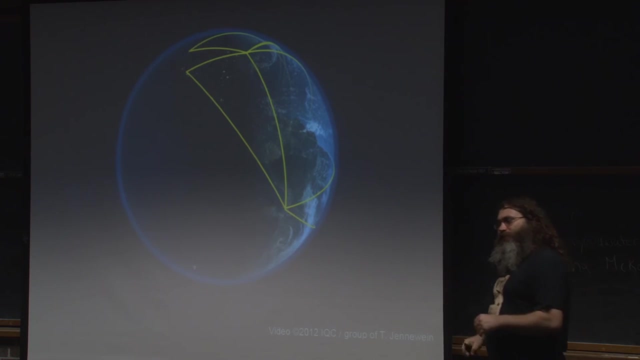 quickly. it covers the globe. a single satellite covers the globe in a big key distribution network and then you can start sealing the key and banking money. so this, this is another research project at this university. these are little space race going on, so we don't know who will be first, maybe. 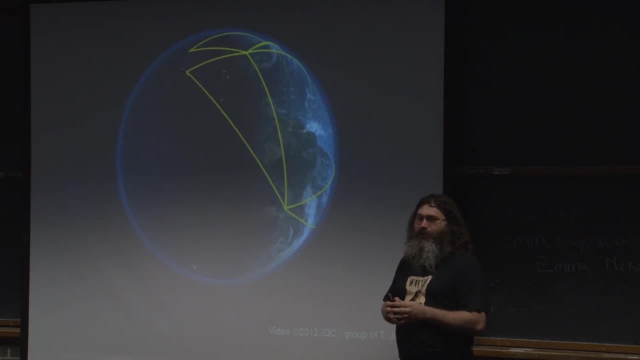 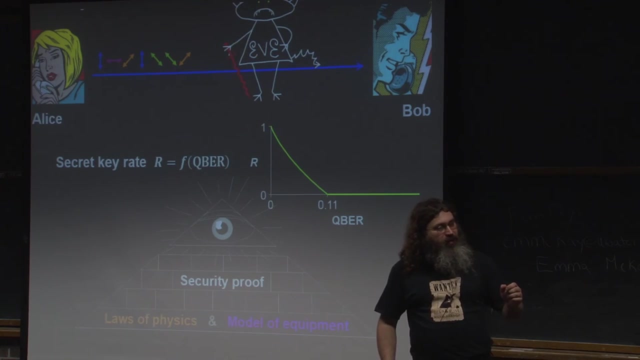 Chinese. they have the plans to launch a satellite in 2016 and I must say they have 20 times more money that than the Canadian Space Agency, but we'll see. so now, how much time do? I left ten minutes, good, yeah, so now we have seen the beautiful. 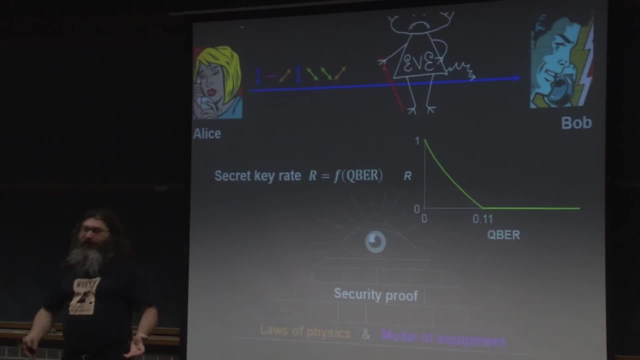 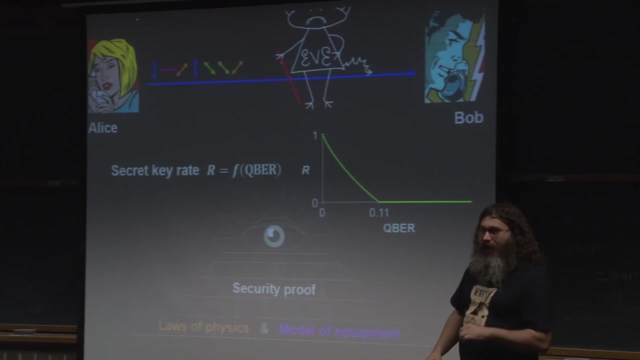 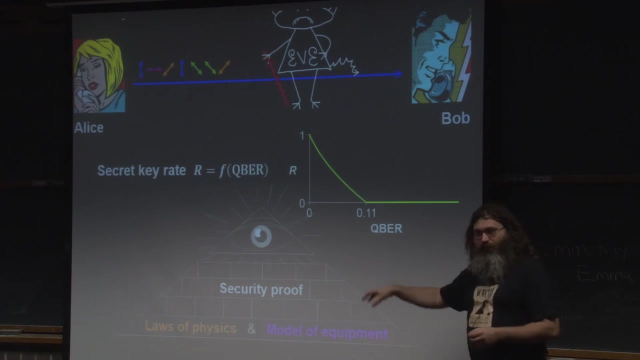 picture how quantum cryptography should work, and we have seen the theory why nobody should be able to eavesdrop on it. now we come to practice. so this is what my laboratory is is doing, and my name is Vadim Makarov. I'm a research assistant professor and my focus at this university is try to break the security. 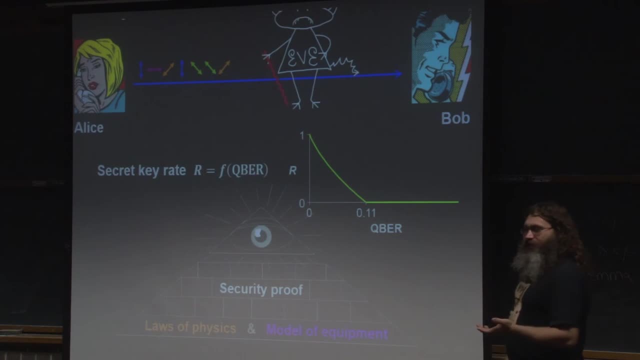 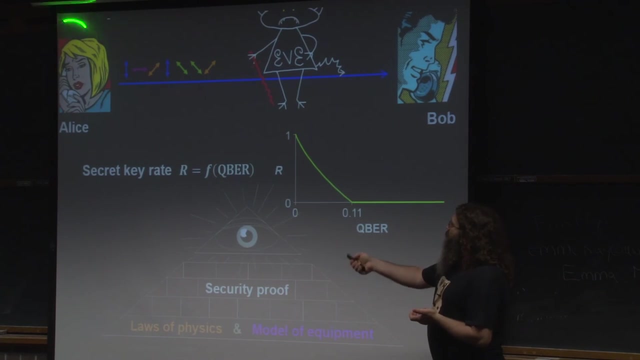 of those systems. how can you break security? the beauty of quantum cryptography is its security model. so you can have. you have Alice, you have Bob, Alice sending to Bob a bunch of quantum states, and here you can have Eve, who is only limited by the laws of physics in what she can do to those quantum states. 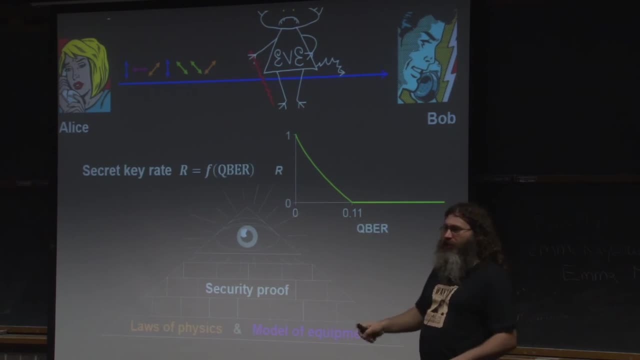 she can have a quantum computer, she can do arbitrary things, whatever is allowed by the laws of physics. to those states that the security model of quantum cryptography consists of three components: first, we have the laws of physics. second component is the model of equipment, the security proof. the security model has a simplified model. 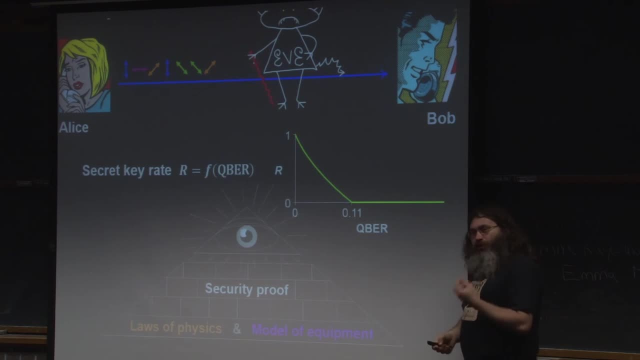 of equipment that alice and bob use, based on those two components: the laws of physics and the model of equipment. the security model proceeds with the third components: security proof. this is a mathematical and logical derivation which starts with those two components and arrives at a security result. the security result says: if alice and bob do the protocol and they measure a single parameter, 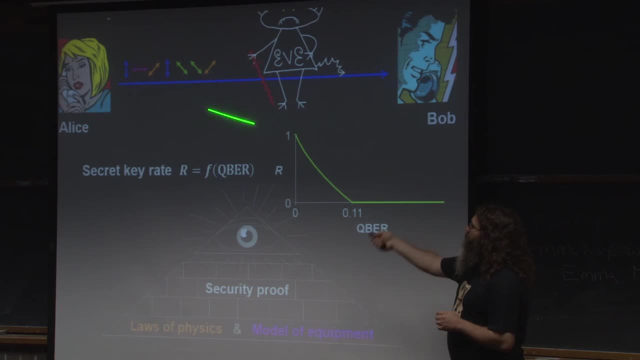 during the protocol, the percentage of eras between alice and bob. then from the value of that parameter they know whether their communication was secure or not. so in the simplest case, they are looking for this percentage of heroes, and if it's above 11 percent they cannot have security. 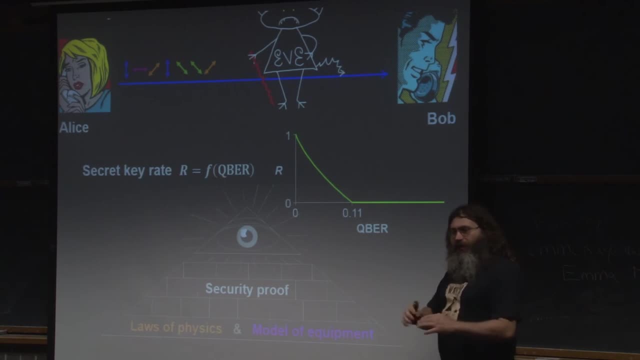 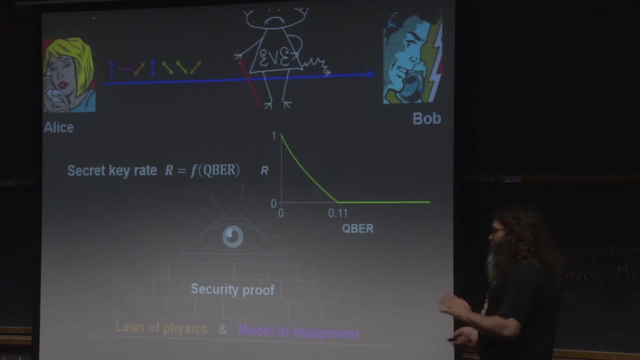 if it's building 11%. they can make a secret key out of this communication: how to break the security model. we can't do anything to the laws of physics. we are not trying to. this is quantum mechanics, the best physical theory we know today. I can't do. 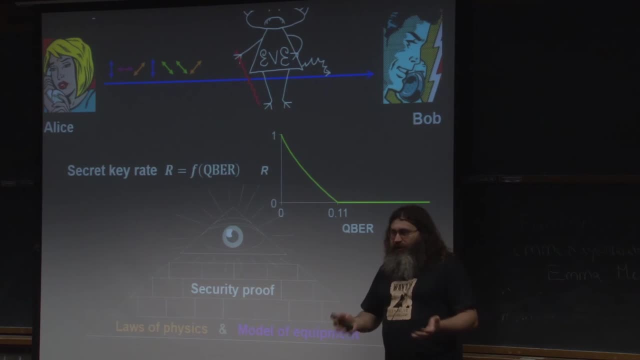 anything to the security proof because we believe it has been examined many times. it's just logic without any holes in it. but there is the model of equipment and all the recent attacks of the last few years have targeted this component. it turns out the real equipment used by Alice and Bob is much 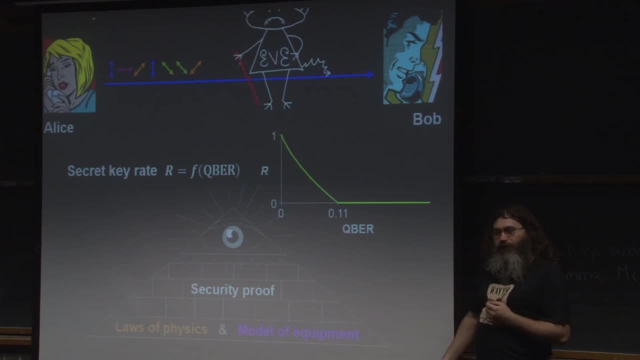 more complicated than the assumptions in the security model. components and Alice and Bob have imperfections. sometimes they behave in a very different way, though the theory requires them to do. Alice and Bob have lots of software, lots of electronics, lots of algorithms, and those are made by engineers. 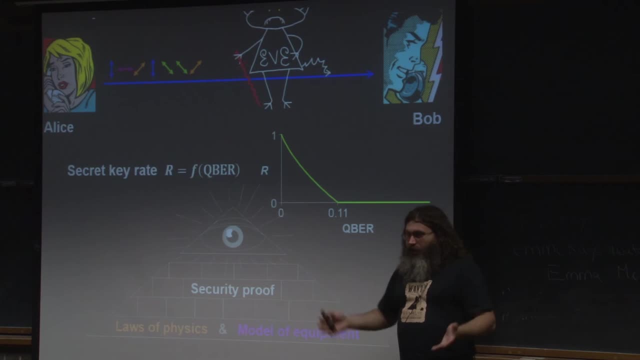 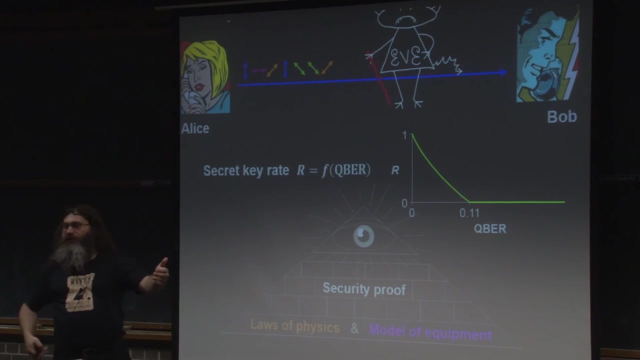 you and engineers make mistakes or very often they don't understand how to build things securely and they don't want to think and they have a deadline to build it by next month and they make something that works, that does the protocol. and if you run it as the engineer as intended, then the protocol runs, but then you 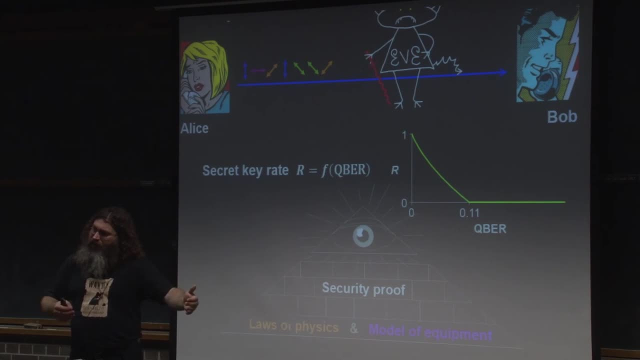 start thinking: how can I do something different and break the security? and very often you find this is the difference between the actual behavior of equipment and the model and based on the difference usually you can construct a working practical attack. so engineers are totally not good at breaking their own. 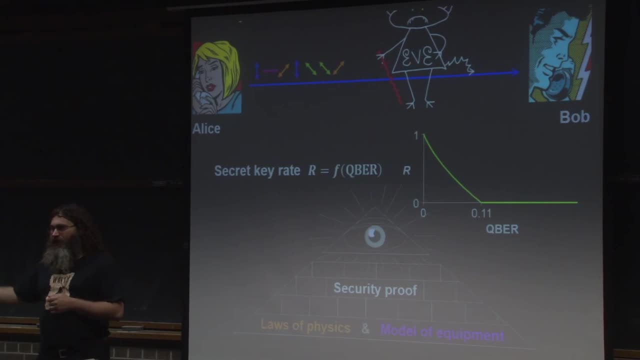 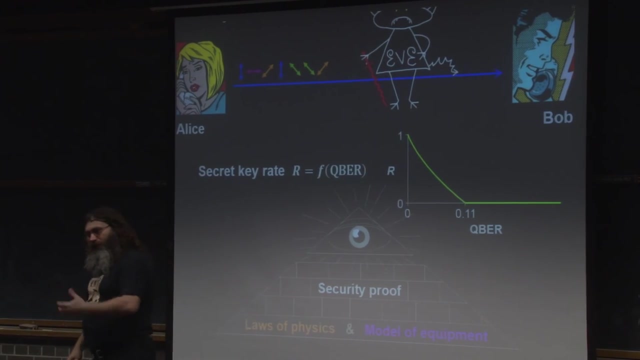 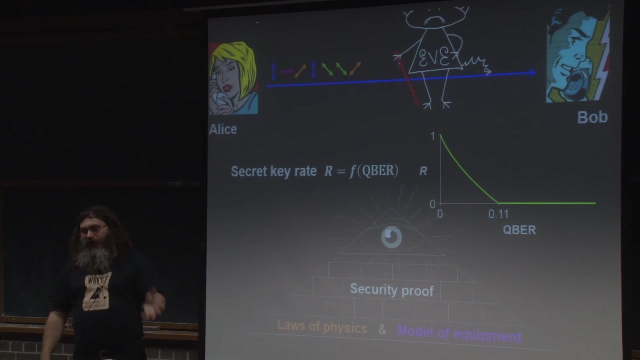 equipment. you need an independent party, an independent hacker, to look for those loopholes. so we have like a job separation. companies make systems and my students break them. we before we try to both build and break and it didn't work very well. either we built well or we broke well but never bought. 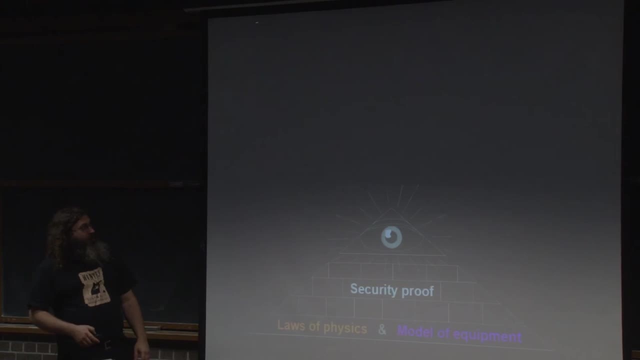 so yeah, so the workflow of working with researchers and companies is the following: we have the cryptographic equipment, the practical implementation, and we hack it. so we find this discrepancy between the model and the actual equipment. we construct an attack, we let them now, we publish it and then 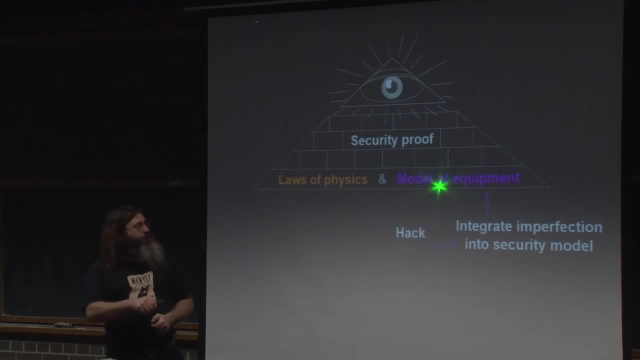 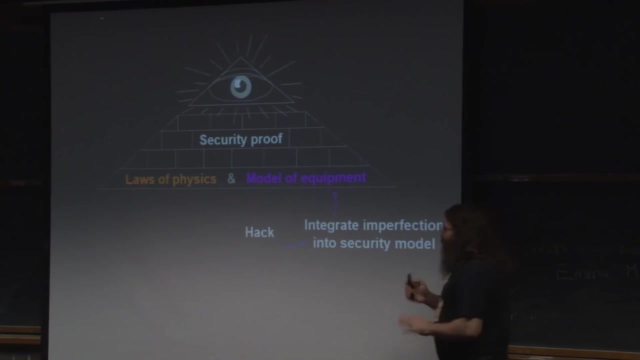 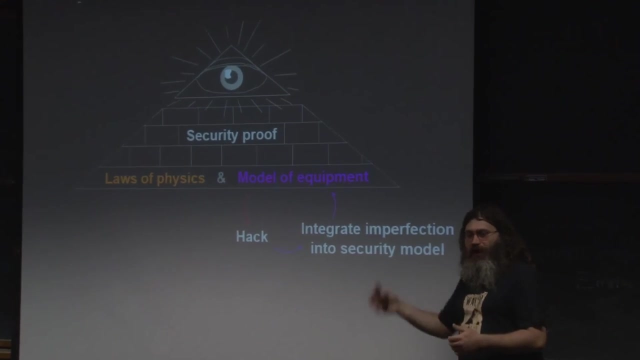 the researchers and manufacturers try to improve their equipment. so either they make a patch or they change the protocol, or they say, okay, there is an imperfection, but we know how much an imperfection it is and we integrate this imperfection in the security proof. we made it an extra parameter and we reduce the amount of key and after that we are. 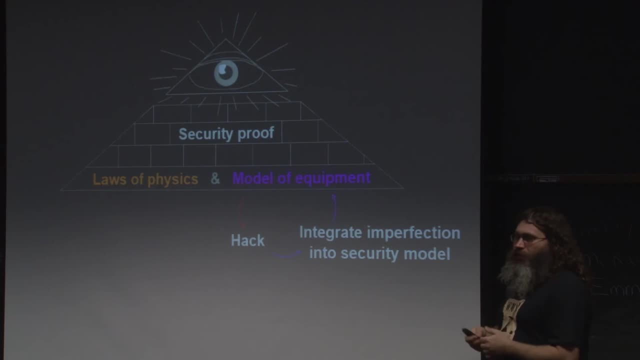 secure. or sometimes they invent a totally different protocol and say: okay, if if you want to do the communication in a totally different way, then this imperfection is still there, but it's no longer a security issue. so all that happens, and then we hack again and they have to change the implementation again. 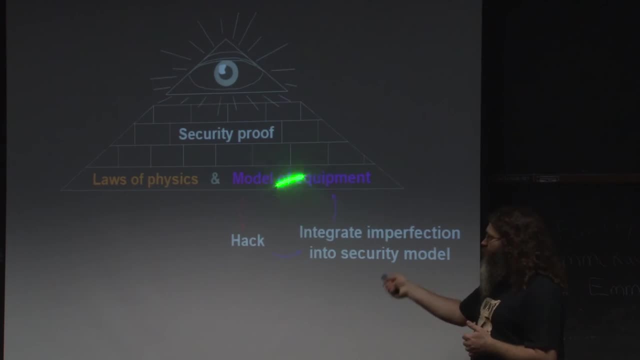 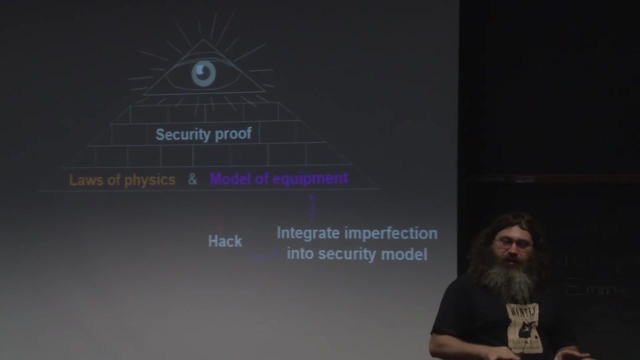 and hopefully after a few. so right now we are in this cycle and there is no shortage of hacks, but hopefully in a few years we will run out of easy hacks and then we will arrive at a pretty secure equipment. so that's, that's the expectation, and I must point out, this is the same thing which happens in classical. 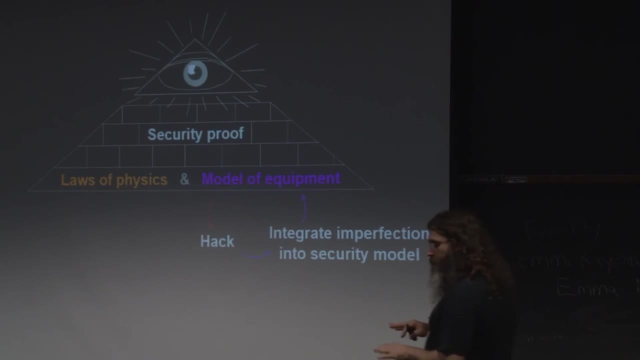 security systems in classical implementations. again you have the implementation issues and we have to watch for things like, for example, in software for stack overflows, for any other type of loopholes, for but, but, but parameter choice. so if you read news several times a year, there's a high-profile attack which says, oh, there was an. 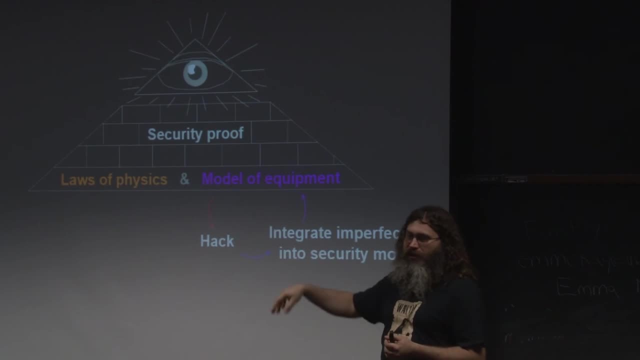 implementation and it's installed to the whole world like a milliard installations and it's crackable and everybody has to do a security update. so this all happens in the classical world as well, and it does happens in the quantum world, but our hacking requires an optical lab, unlike somebody in the 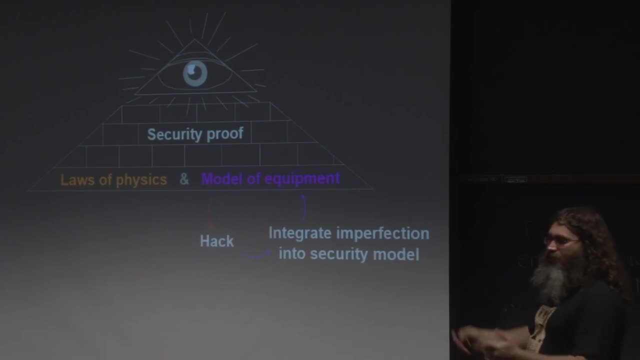 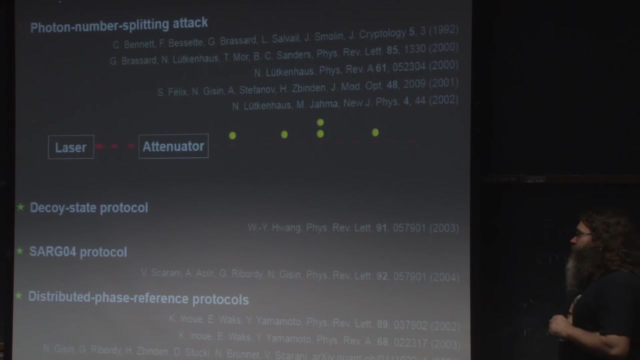 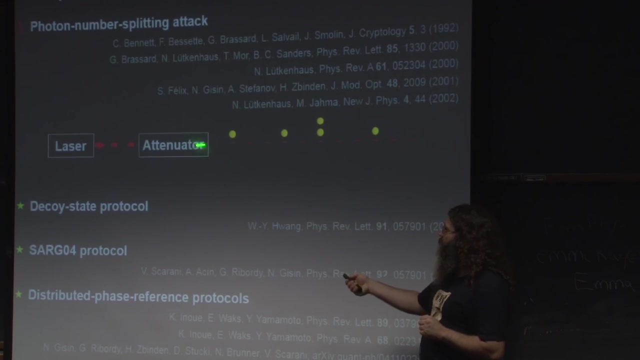 basement, who can use their skills and the computer to crack software. so I will give you one or maybe two examples of practical attacks. so one example of practical imperfection is what kind of photons you are sending out of your, your sender. so far we assume those should be single photons. but 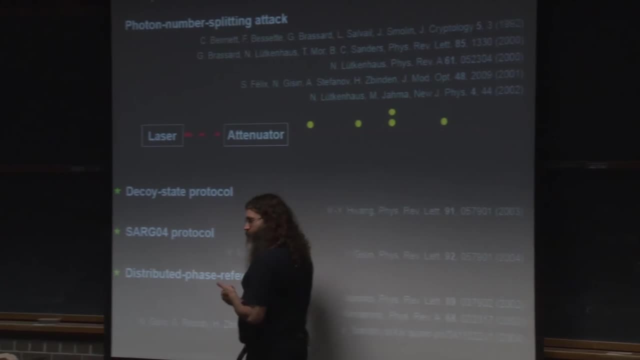 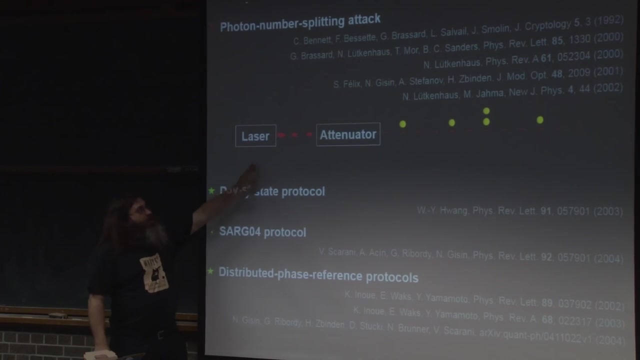 single photon sources are difficult, they are not very practical. they exist but it is much easier, instead of a single photon source, to use just a laser and put an attenuator after the laser. and when you do this, out of your laser sometimes they come empty pulses that contain no photons. and sometimes, if the you, if you, 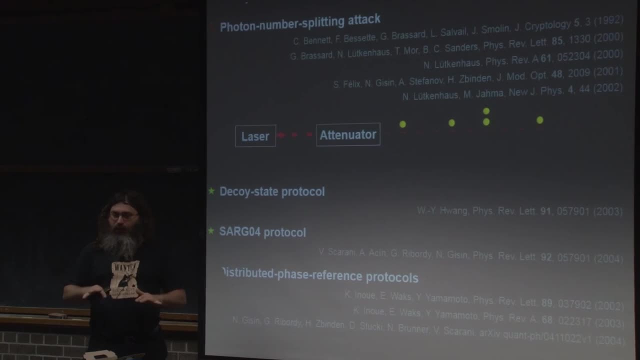 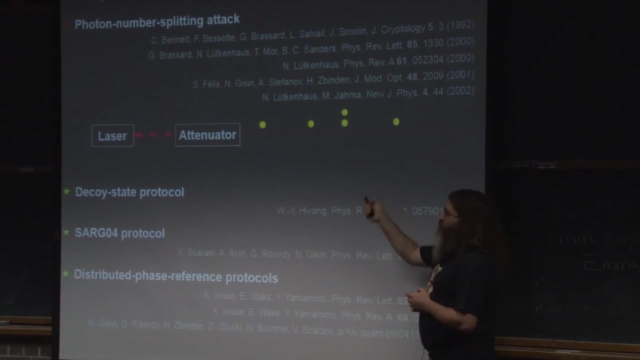 attenuate the pulse heavily enough, so on average you have less than one photon. on average, then most of your pulses will be empty and some pulses will contain one photon. the problem is sometimes, with a smaller probability, your pulse will contain two or more photons and that is a security problem. Eve can take measure the number of photons she is. 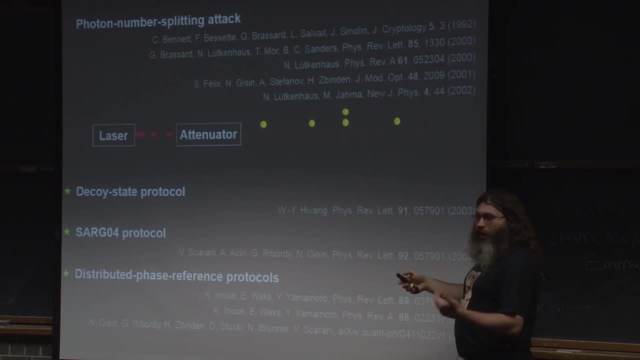 allowed by quantum mechanics to do a photon number measurement. and now, how many? zero, one or two. and if she finds two, those are prepared in the same polarization state. right, she can take one photon and store that photon in a quantum memory. another funny things that physics allows and we are trying to. 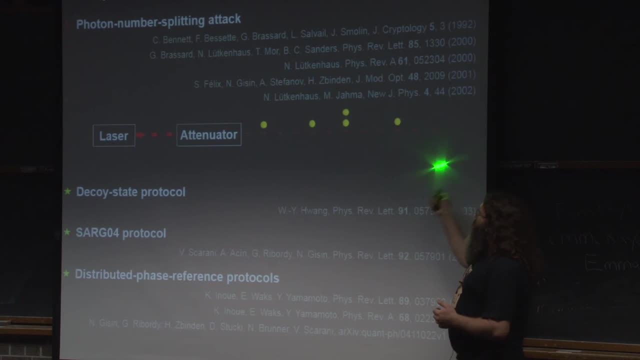 build it, but let the other photon go to Bob. so Bob detects dot photon and Alice and Bob announce the encoding basis. then Eve takes her stored photon in the memory and measures in the same basis and Voila, she knows this bit value. so the multi photon emission of the 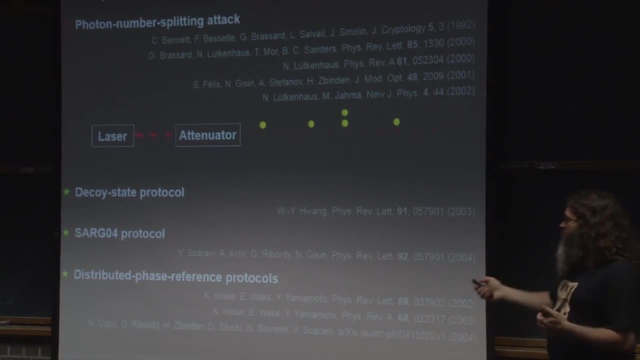 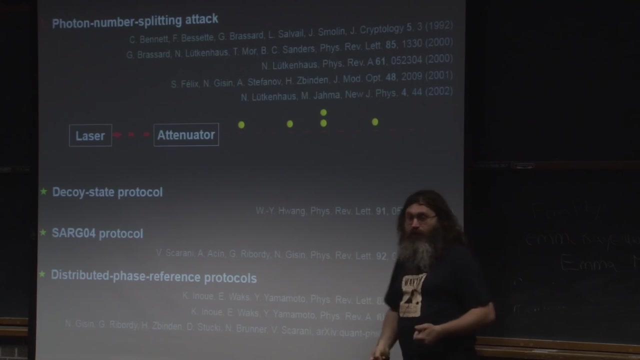 from the source is a practical problem if you use this type of source- and those sources are much more convenient than the single photon sources- you can build this out of a laser and attenuator- standard telecom components in something like a laser. laser at us, Yes, so sense, sense. 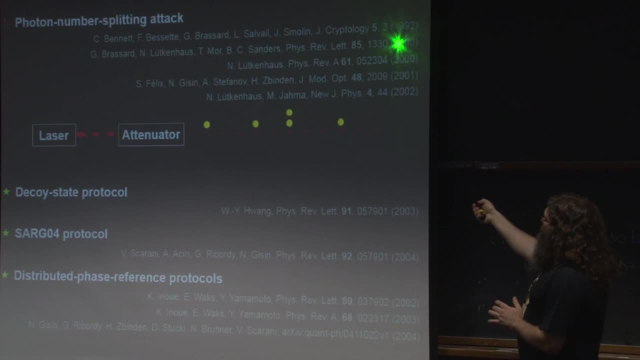 that they will be able to scolded and that the Reverb operation, when you want to actually be able to do a distance regularity unlearning problem and then you'd be able to calculate något, to able to Do a pointer retroação per goes. 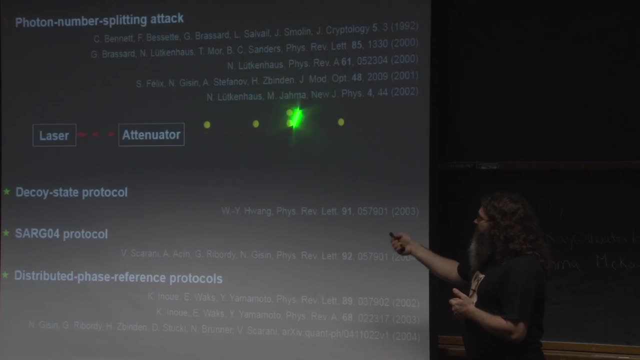 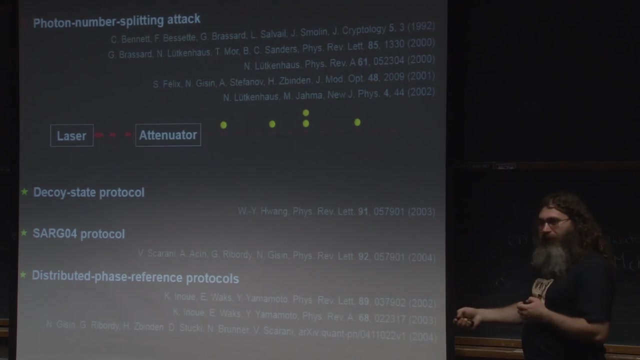 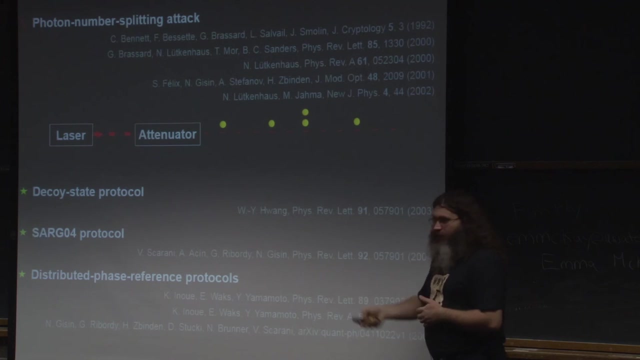 in always the same, in 3 it and incorporate it inside the security model. and now everybody, almost everybody, uses laser and attenuator and those schemes are secure, even though they often emit two or more photons, because the protocols are modified and they run in a clean way. taking this imperfection into account, and if you 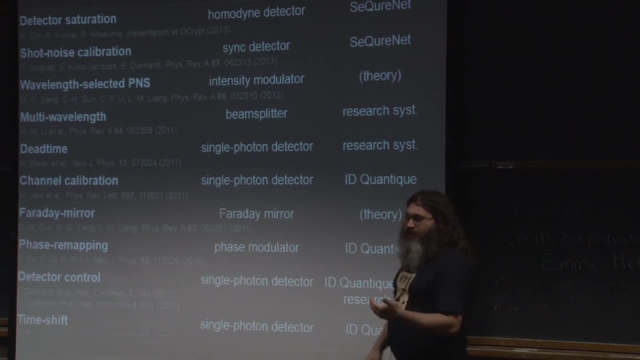 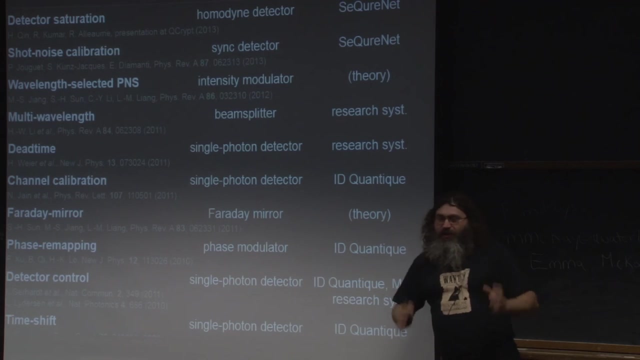 look at what's happening, really happening in this research and manufacturing community last few years. you see many attacks, practical attacks, targeting that kind of component imperfections, and this is a partial list, not very much updated. this year they have been three new attacks. I didn't have time to write them on the top of the list and you see that the different 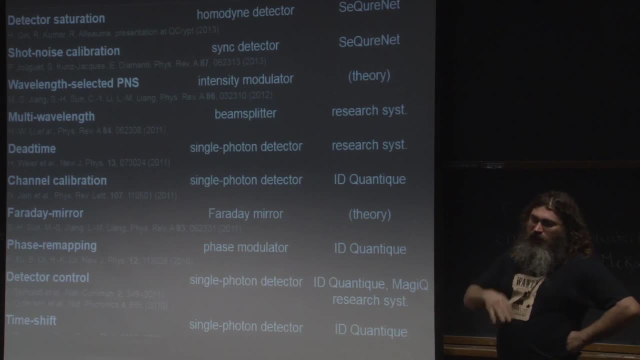 attacks and their groups working all over the world: Canada, Europe, China, Asia. they target imperfections, imperfections, different imperfections in implementations, different components, detectors, modulators, beam splitters, mirrors and two different types of detectors. Most of the attacks are verified on Commercial equipment and some of them are verified on research equipment. So just in this table you have three different commercial systems. 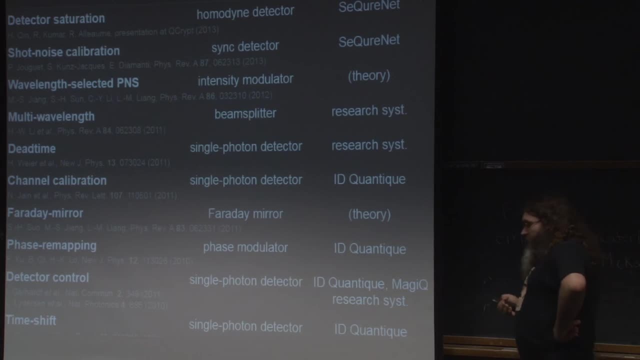 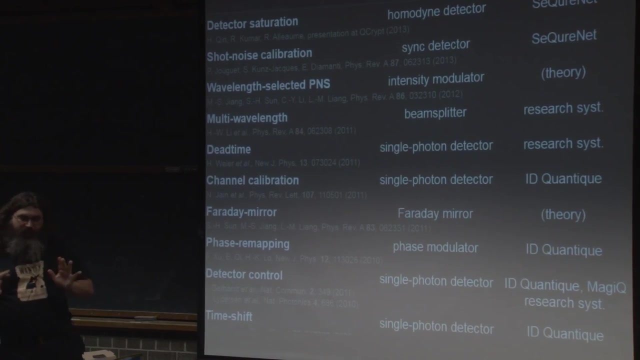 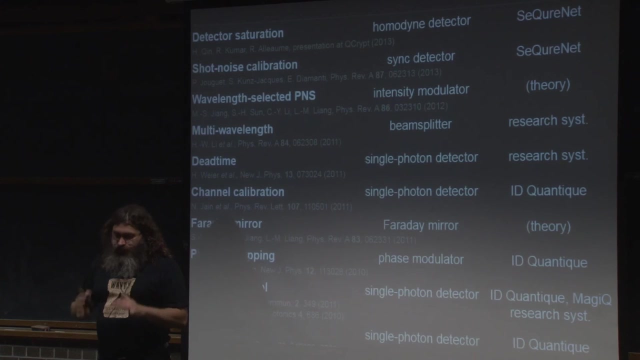 So the different attacks apply to different systems. so this process is happening and and The attacks. but what makes me optimistic is that every time there is an important attack in a few years, The manufacturers and the researchers come up with a good, clean counter measure to incorporate the attack inside the security proof. 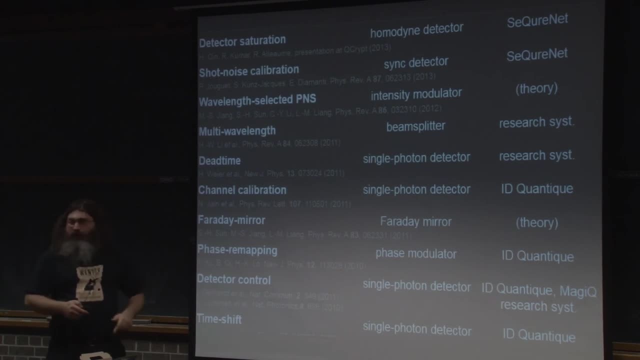 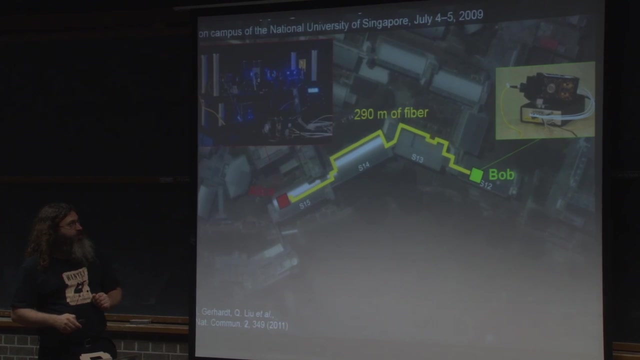 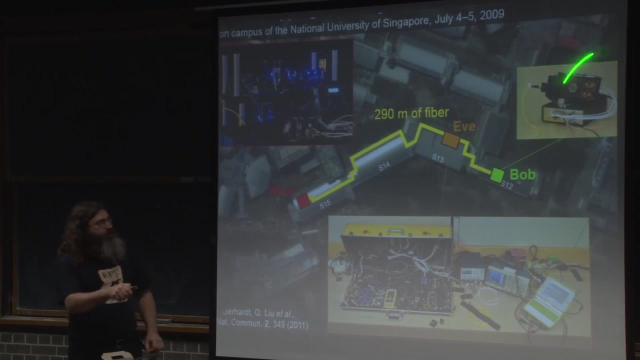 So I had another example of attack. I don't have time I will skip a few slides to leave time for questions. So that was another attack we did. Yeah, so that was Very good eavesdropping. So just to show you the slide, we found another imperfection in another part of the system in single photon detectors. 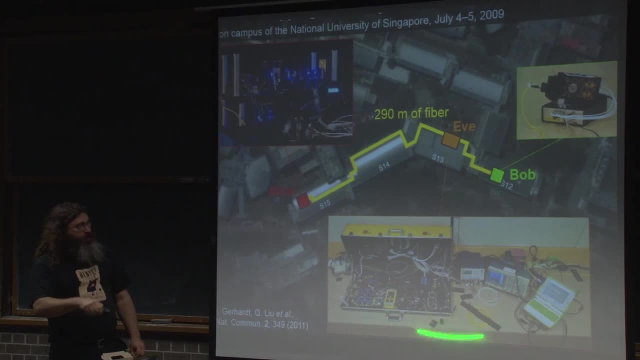 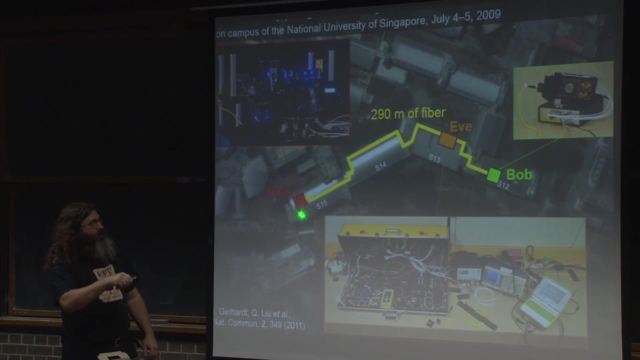 And we did an eavesdropping where we built the actual eavesdropping. So this was our hiking suitcase five years ago where we installed it on the line between Alice and Bob and this computer and suitcase had the full secret key information. Alice and Bob did not suspect anything. they generated the same key and they didn't notice anything wrong. So that was.